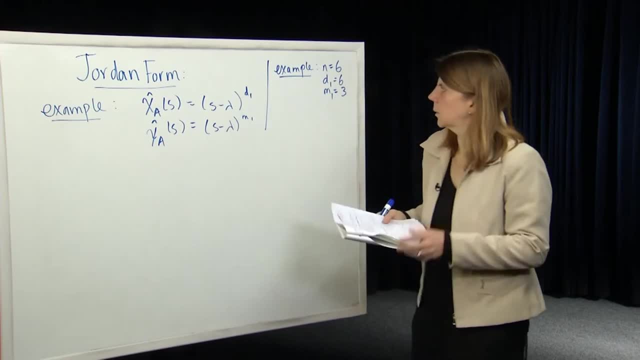 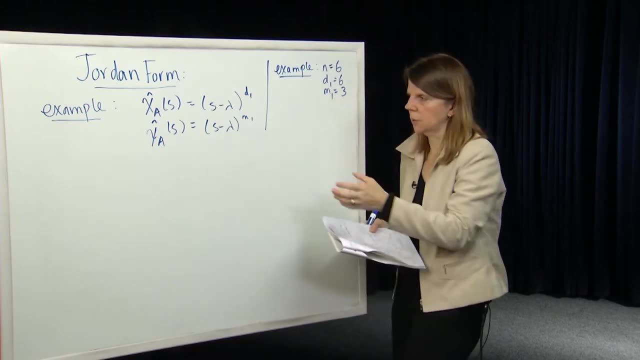 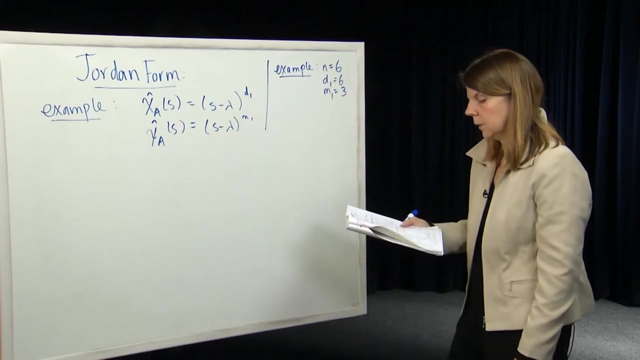 that m1 is equal to 3.. Okay, so we've got a minimum polynomial. We have, as introduced from the last module, the largest Jordan block is of size 3, associated to that eigenvalue at lambda. Okay, so what does this tell us? Well, it. 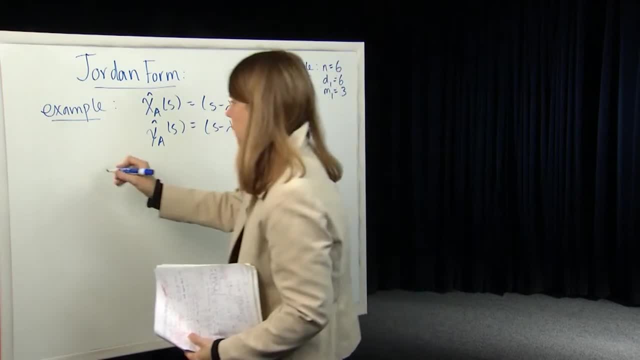 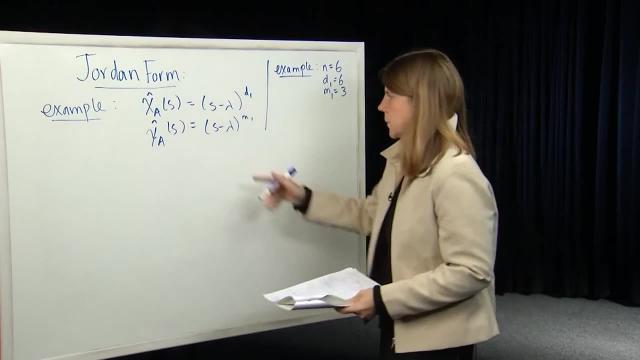 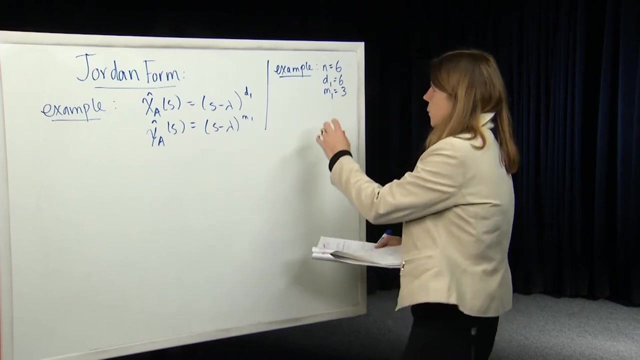 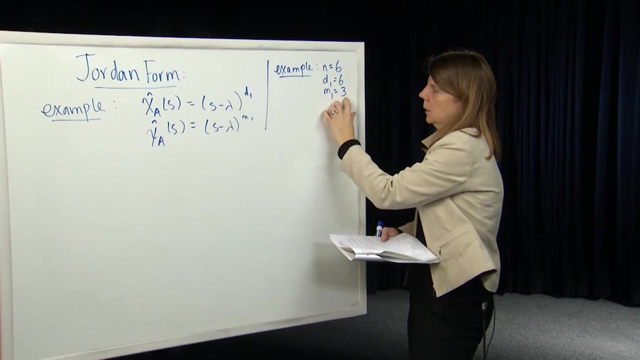 tells us a couple of things. So in this example we're going to suppose that we have again. it's just one eigenvalue which is repeated at lambda, and we know that the difference between the dimension of the matrix A and the largest Jordan block is 3.. Okay, so that tells us that we could have 2 Jordan. 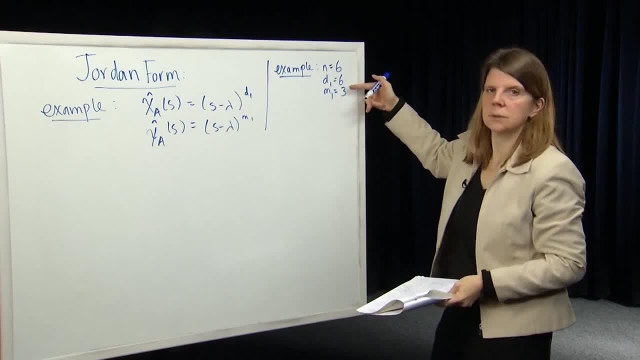 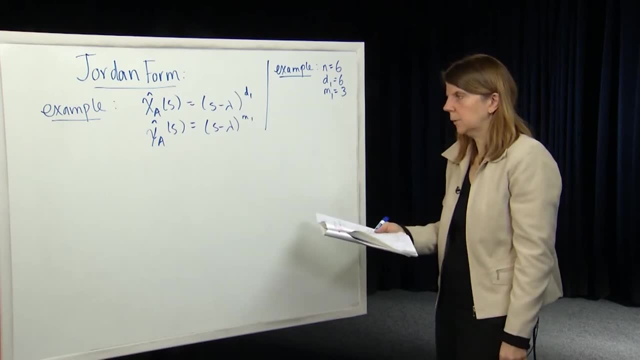 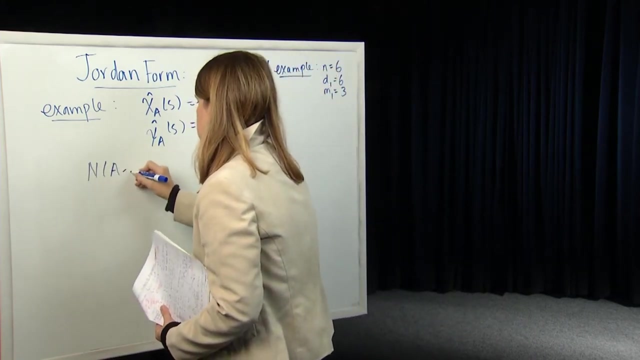 blocks of size 3, or we could have one Jordan block of size three and a Jordan block of size two and a Jordan block of size one to get up to the dimension n. Okay, so in this example, let's suppose that the null space of A minus lambda- I okay, so remember this- is: 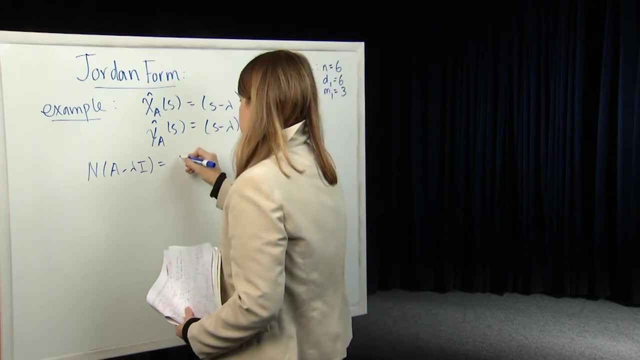 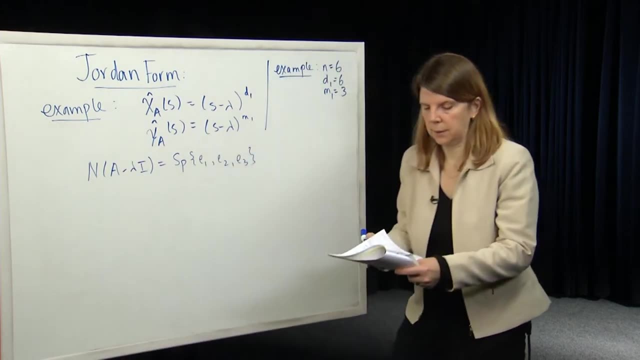 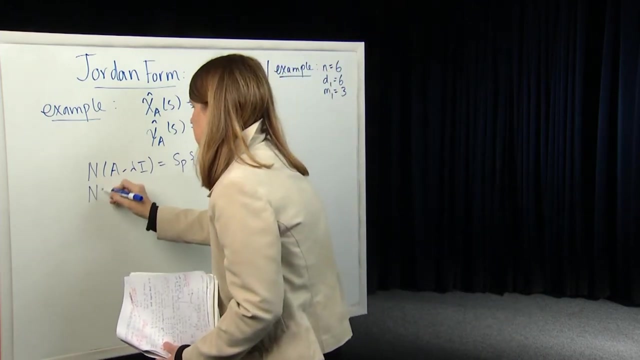 how we compute the eigenvectors of the matrix is: is dimension three, so it's the span of three eigenvectors: e1, e2 and e3. all right, so this is part of the example. let's suppose that the null space of A minus lambda I squared is: 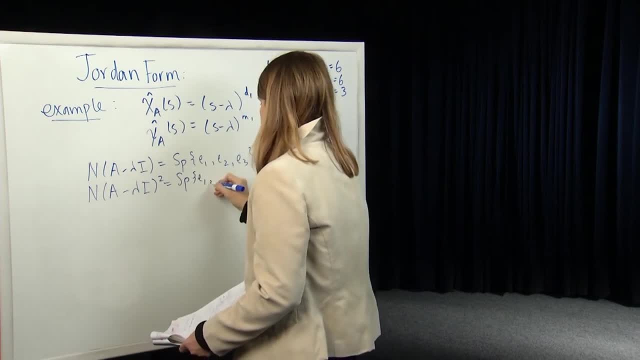 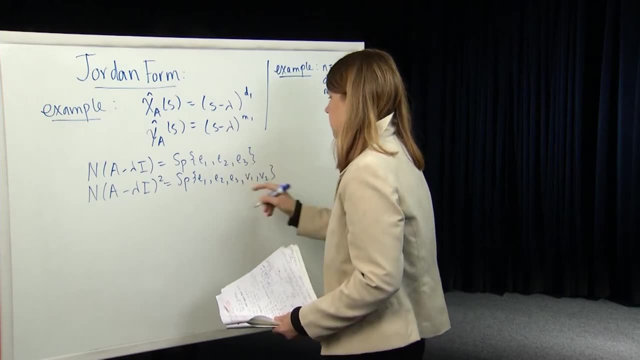 equal to. so it has to contain the null space of A minus lambda I. so it's already got those three eigenvectors in it, but suppose you can add two more linearly independent vectors into that null space, and that's some v1 and v2. 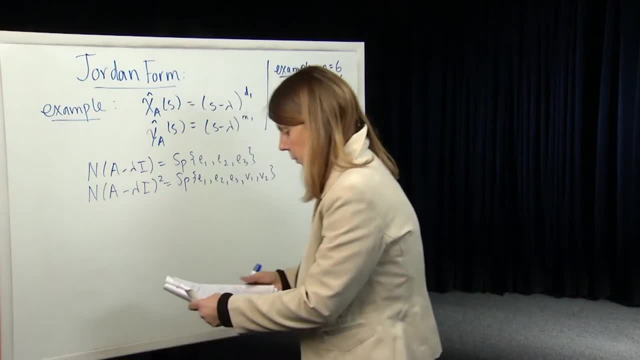 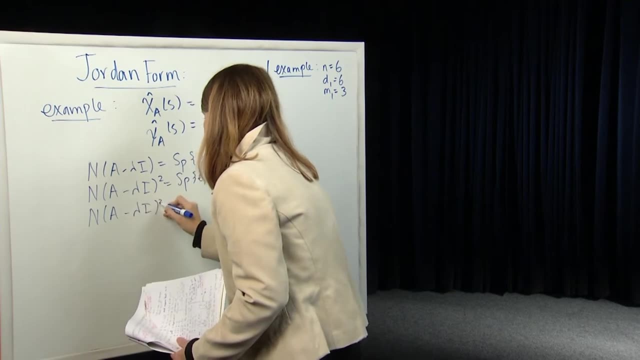 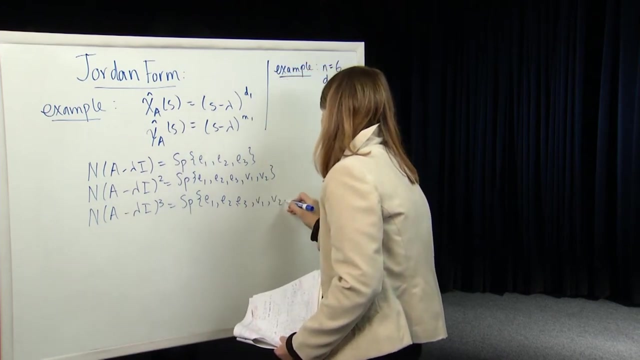 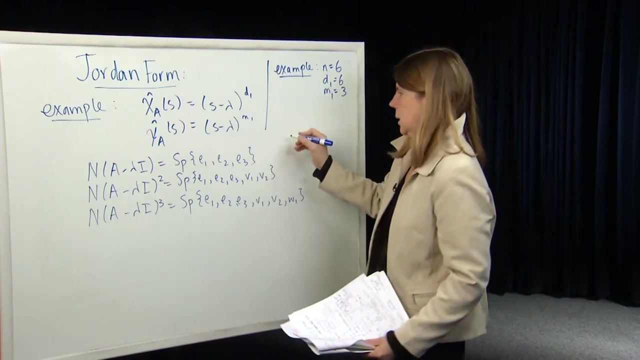 we'll call them those, and then let's suppose that then the null space of A minus lambda I cubed. you finally get the six dimensions. so it's e1, e2, e3, v1, v2, and we'll call the third one W or the sixth one w1.. Okay, so basically what this is saying is: so what? 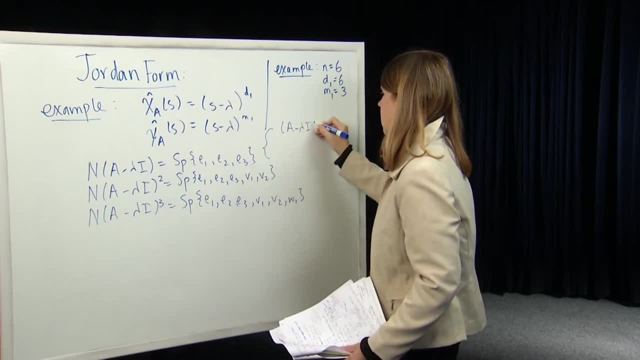 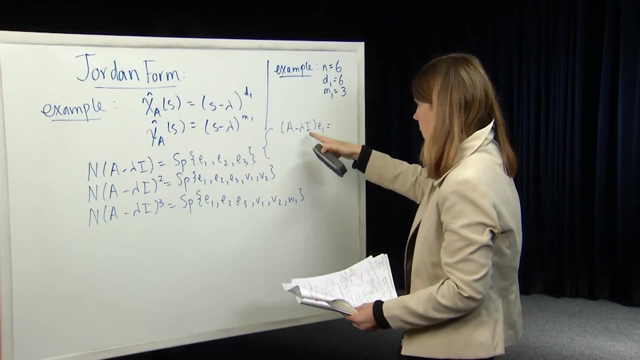 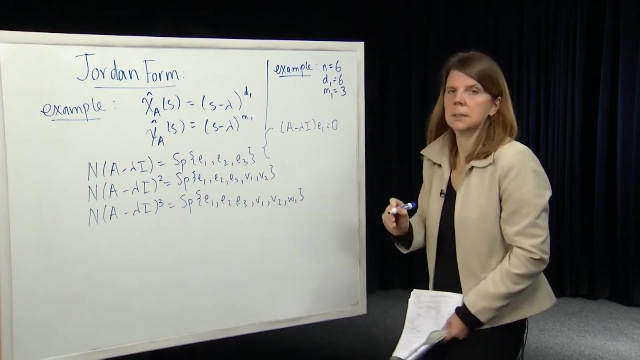 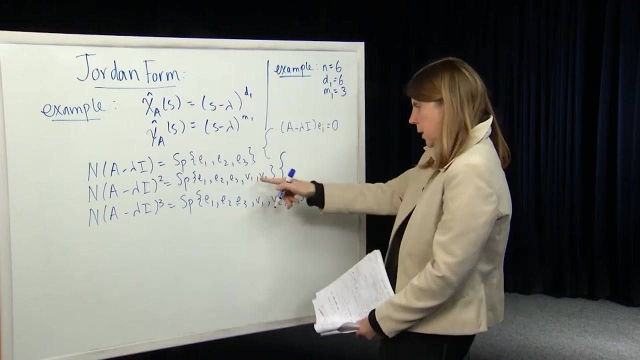 this one is saying is A minus lambda I e1 is equal to or? sorry, yeah, that's right. a minus lambda i e1 is equal to 0, a minus lambda i e2 is equal to 0, and a minus lambda i e3 is equal to 0.. What this is saying is that v1 and v2 are. 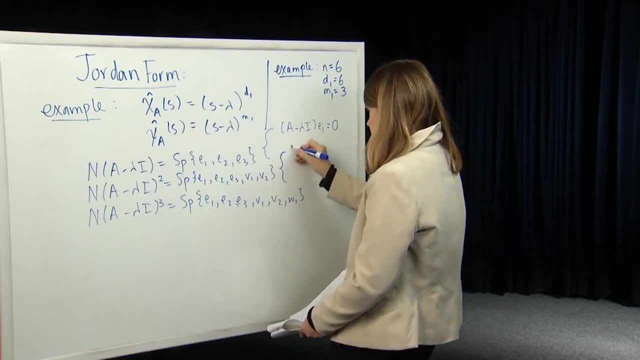 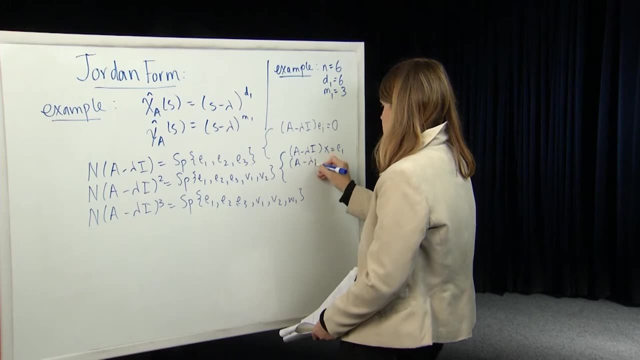 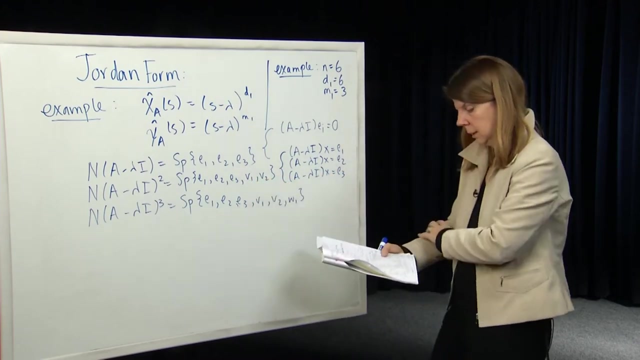 linearly independent solutions of the following equations: a minus lambda i x is equal to e1, a minus lambda i x is equal to e2, and a minus lambda i x is equal to e3.. So you take those three equations and there are two linearly independent solutions, v1 and v2,. okay, So that. 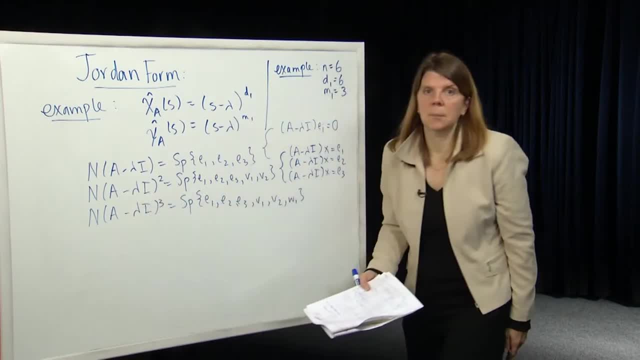 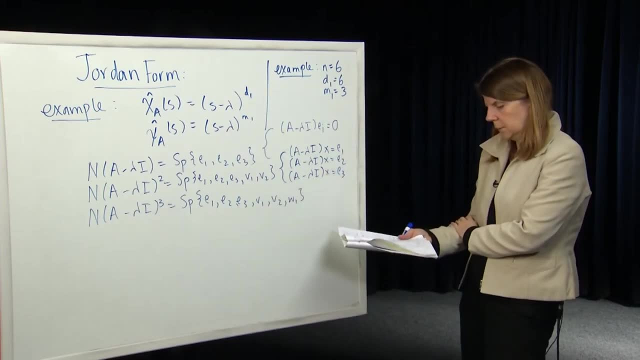 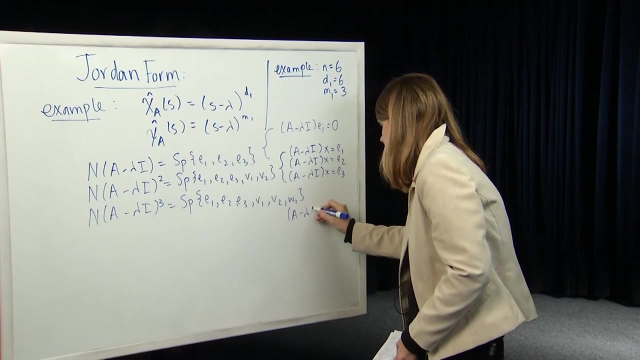 tells us that v1 and v2 belong in the null space of a minus lambda i, And then finally, a minus lambda i- cubed allows us to complete up the null space. So here we have that w1 is a solution to a minus lambda i- x is equal to v1, or a minus lambda i- x is equal to v2.. 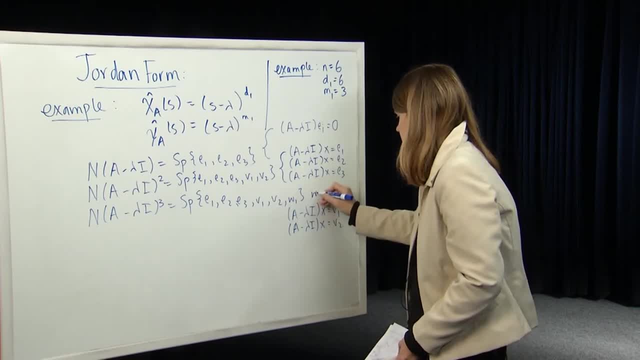 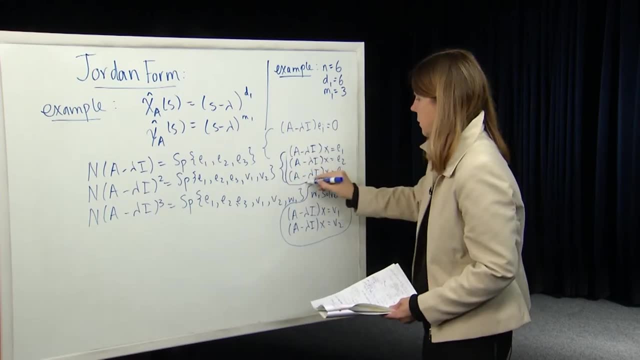 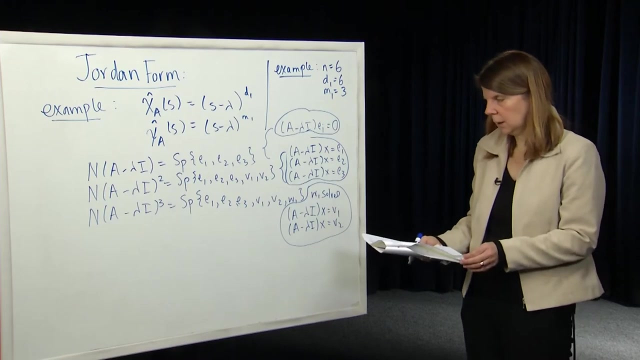 Okay, so that's where w1 solves one of those. Okay, so we solve these equations to get the vi's, we solve these equations to get the ei's and we solve these equations to get the w1.. Okay, so, let's, let's now write out what we. 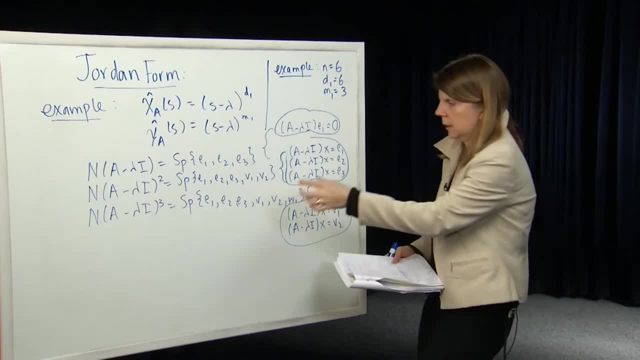 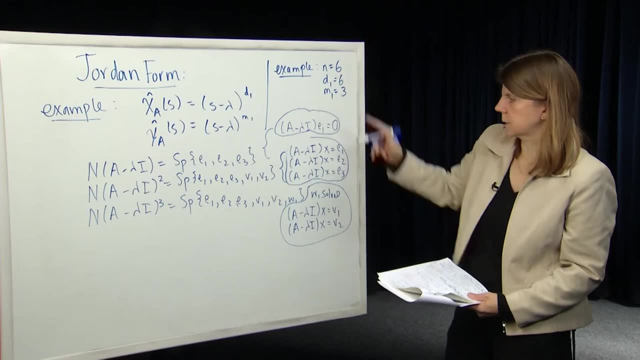 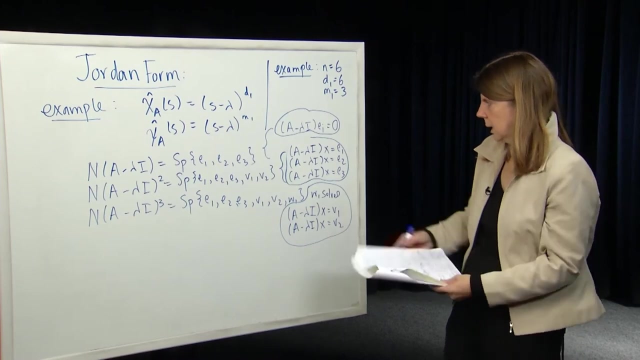 have. Okay, so we have that. the span of the ei's, the vi's and the w1 gives us r6, because we have a six dimensional system and there's six vectors in it, And so now we can write out these equations. Let's actually write these out in terms of our eigenvalue. 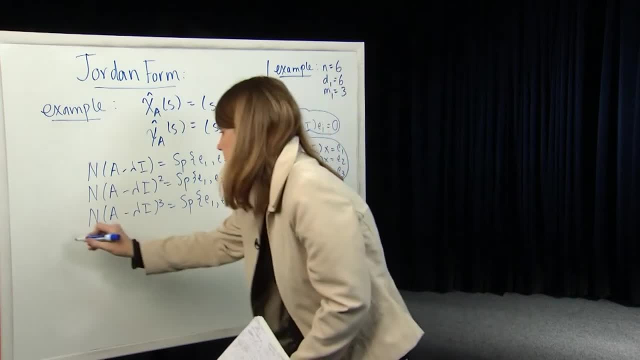 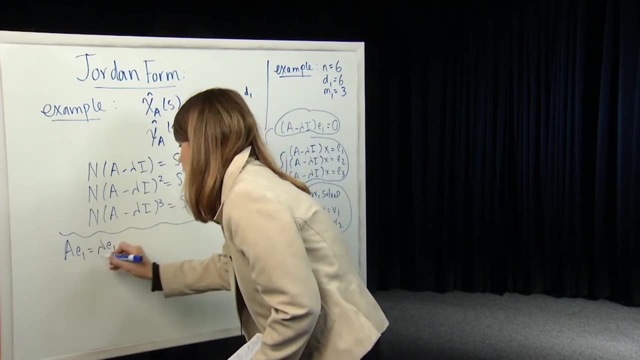 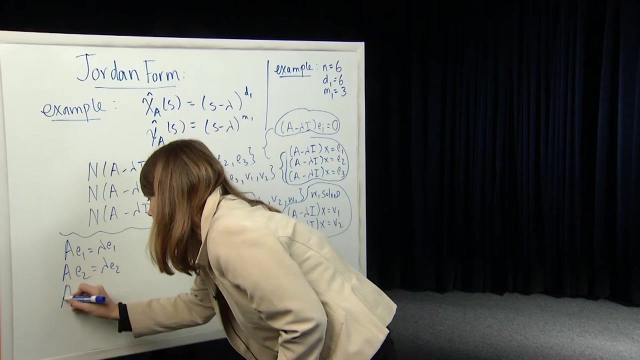 eigenvector notation. So we have that. so let's just sort of summarize: We have that a E1 is equal to lambda E1,, a E2 is equal to lambda E2, and a E3 is equal to lambda E3.. And now these equations here: 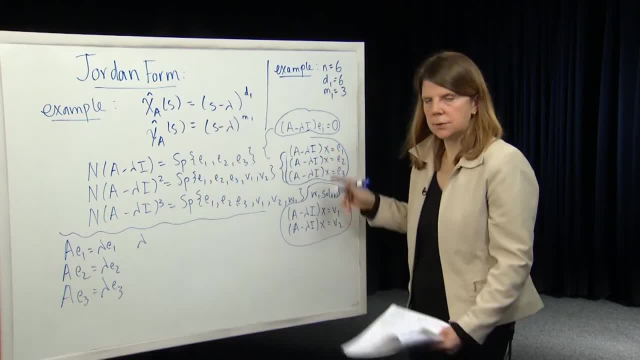 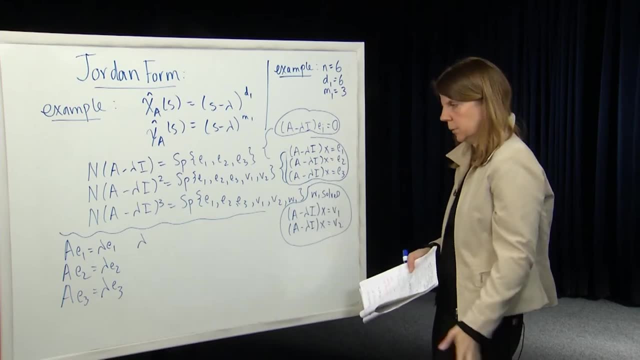 give us A. so let's suppose, without loss of generality, that V1 and V2, they solve these first two equations when the right-hand sides are equal to E1 and E2.. So it's without loss of generality because the structure would be similar. 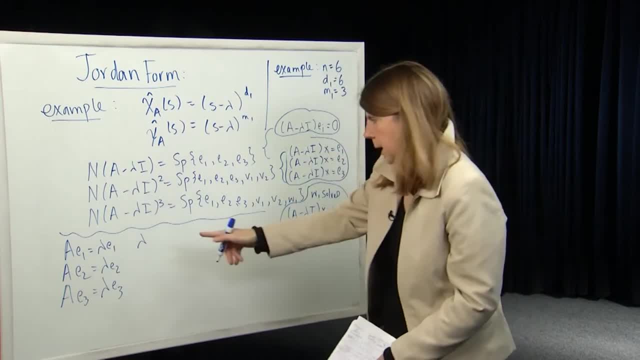 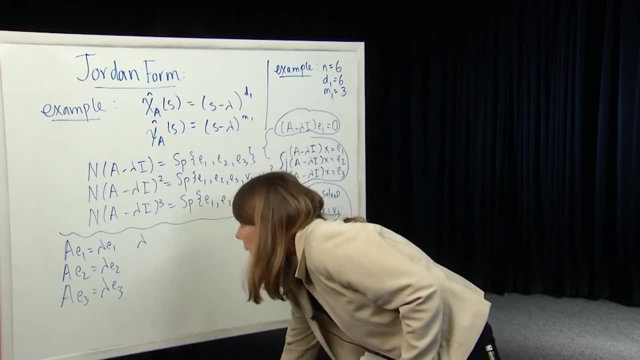 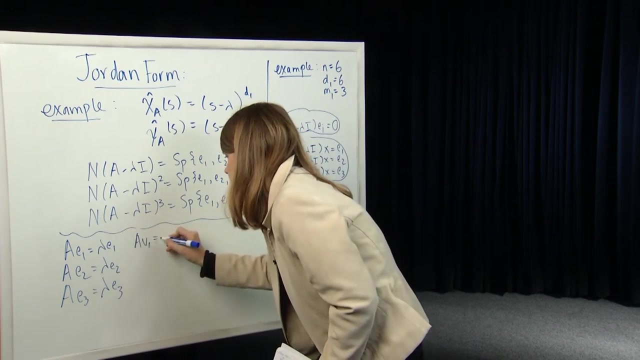 if it solved these two equations or these two equations. But what we have? if the V1 and V2 solve these two equations respectively, then we have that AV1, so we're gonna follow on from these equations here. AV1 is equal to lambda V1 plus E1.. 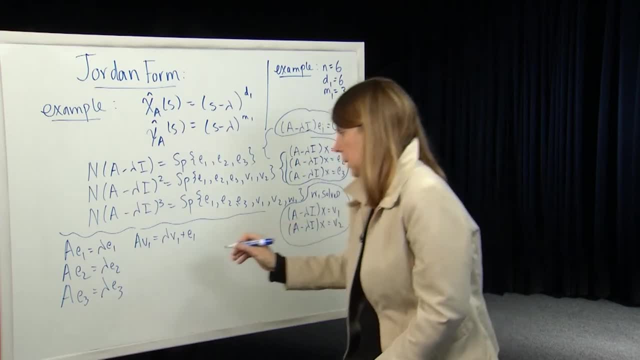 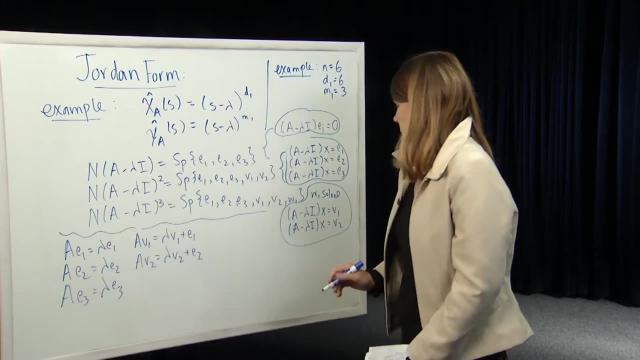 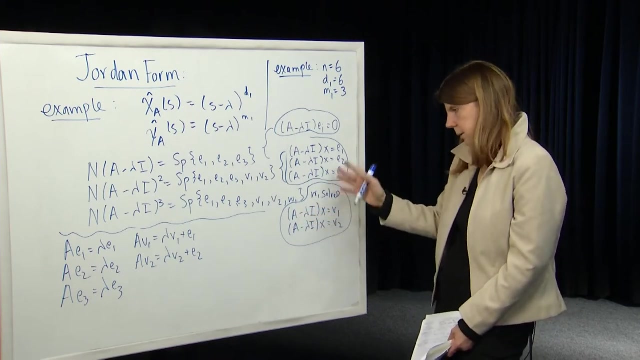 Okay, that comes out of this equation here. And similarly AV2 is equal to lambda V2 plus E2.. And then let's suppose, without loss of generality, that W1 solves this first equation here. It could solve the second, and again it would be similar. 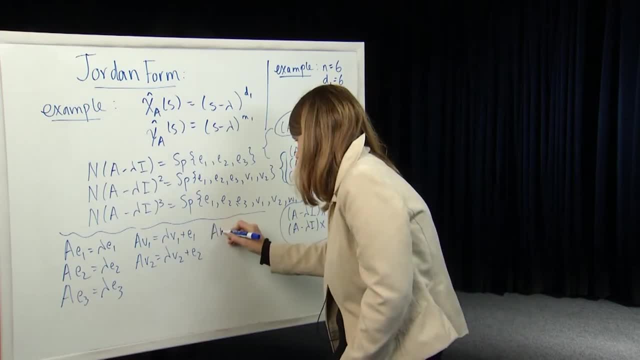 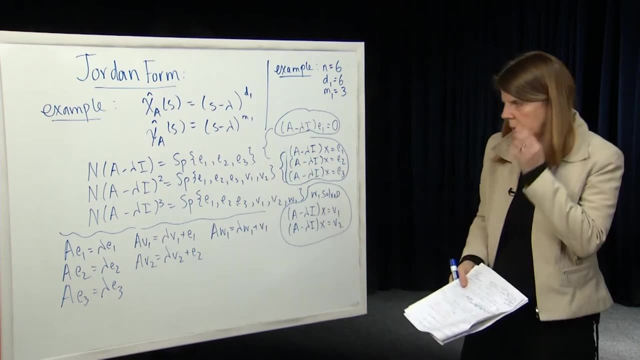 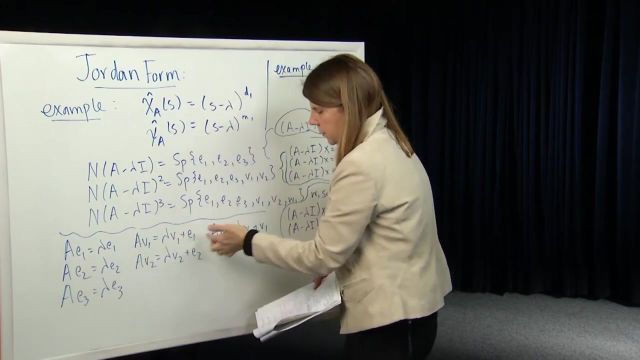 but let's just suppose it solves the first. So we end up with: AW1 is equal to lambda W1 plus V1.. Okay, so that comes out of this equation here. So we have these six independent vectors: E1, up to E3, V1,, V2, and W1,. 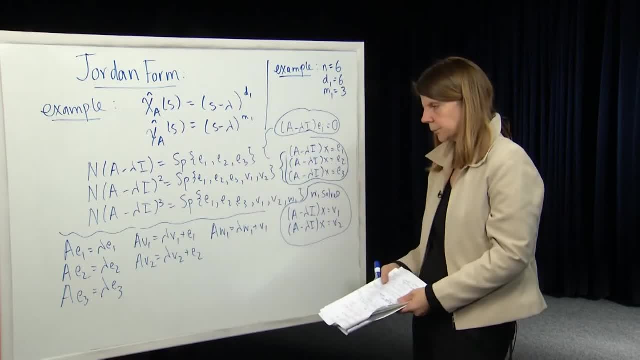 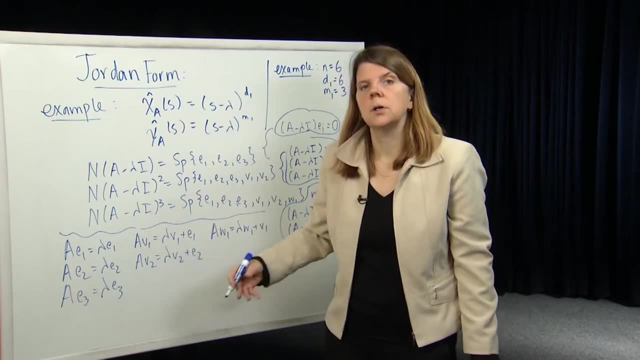 which solve these equations. here. The EIs are eigenvectors of the matrix A, The VIs are called generalized eigenvectors of the matrix A and the VIs are called generalized eigenvectors of the matrix A. The VIs are called generalized eigenvectors of the matrix A. 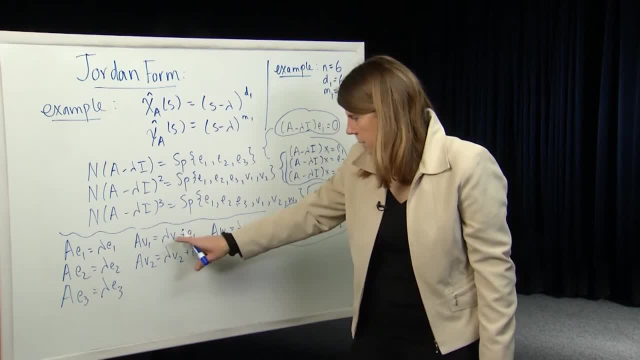 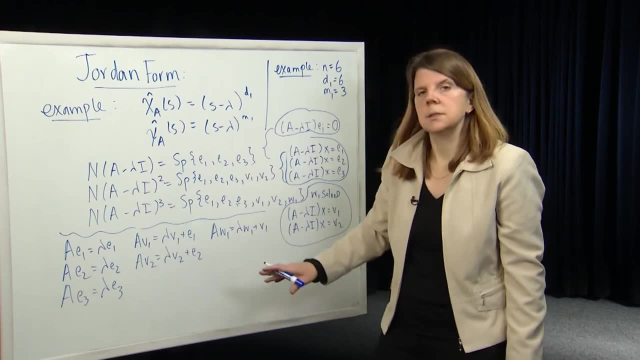 The VIs are called generalized eigenvectors of the matrix A of degree one because the equation they solve of degree one, because E1 and E2 themselves are eigenvectors. W1 is called a generalized eigenvector of the matrix A of degree two. 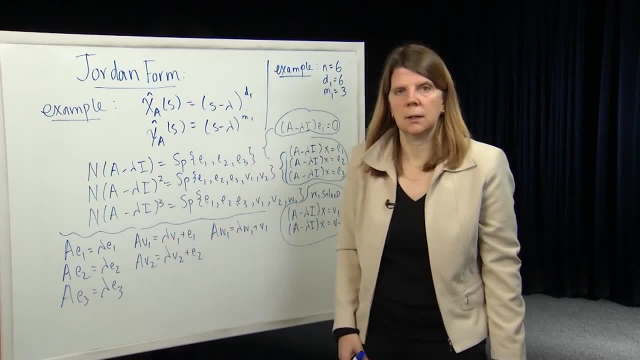 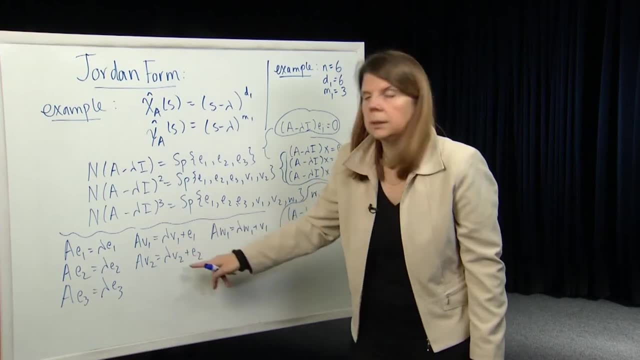 because V1 is already once removed from the eigenvector E1.. Okay, so we have three eigenvectors and three generalized eigenvectors. They're all linearly independent from each other. Okay, so now let's consider okay. 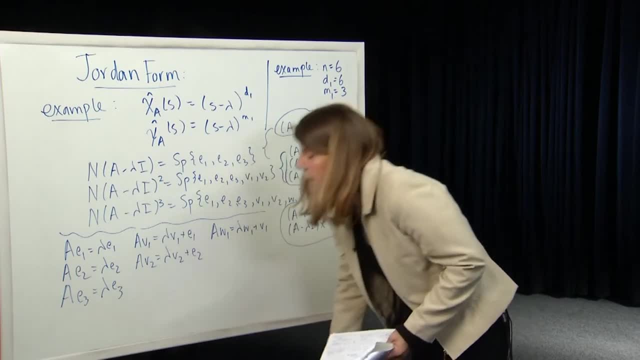 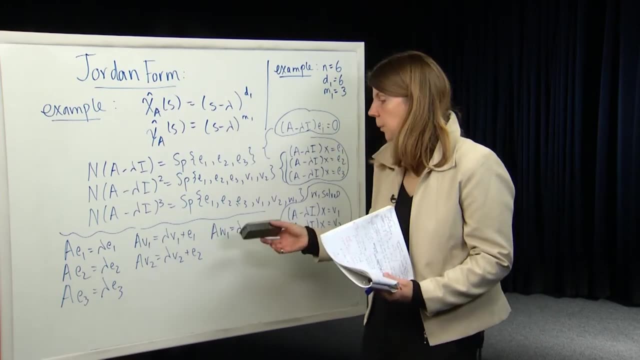 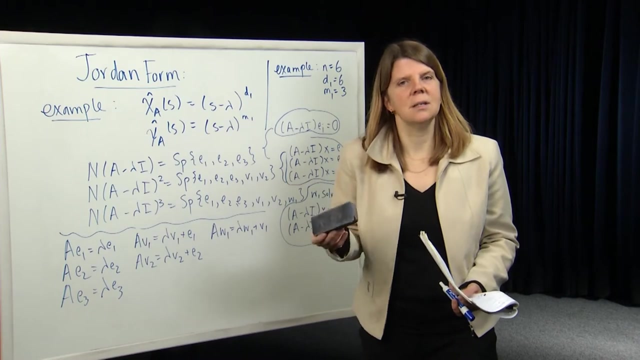 let's consider constructing a similarity transform in a similar way as we did for the diagonal form. We don't have six independent eigenvectors, but we have six independent eigenvectors and generalized eigenvectors, So we'll use those in the column of the matrix T inverse. 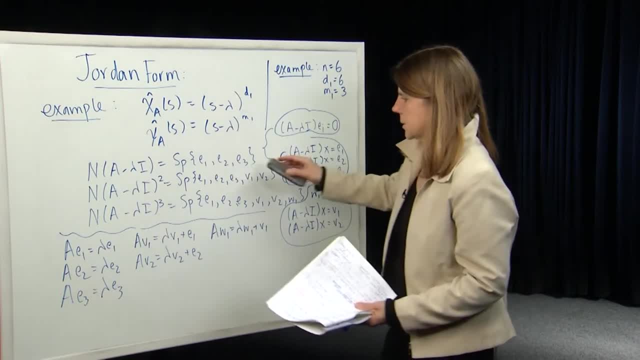 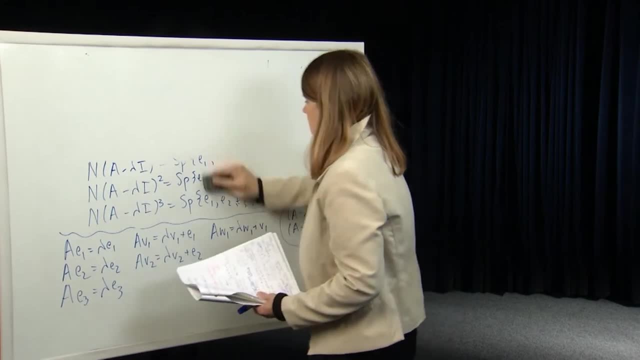 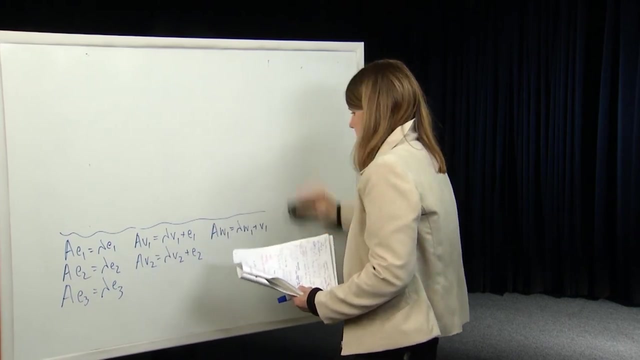 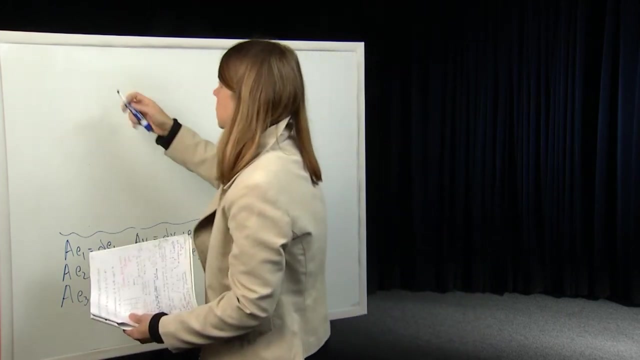 which we use in our similarity transform, Okay. so again, this is just an example, but it's an example which illustrates how we construct a Jordan form. Okay, so I've got my six equations there, Okay, so now I'm going to construct a matrix: T inverse. 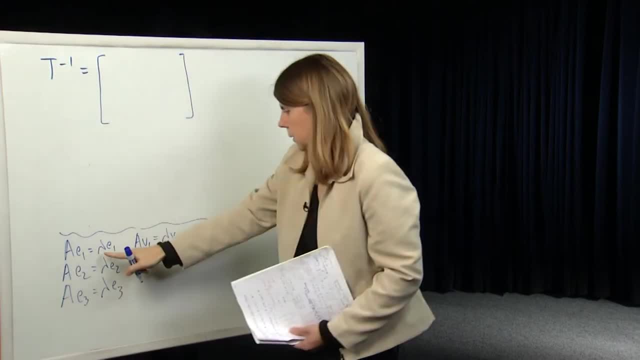 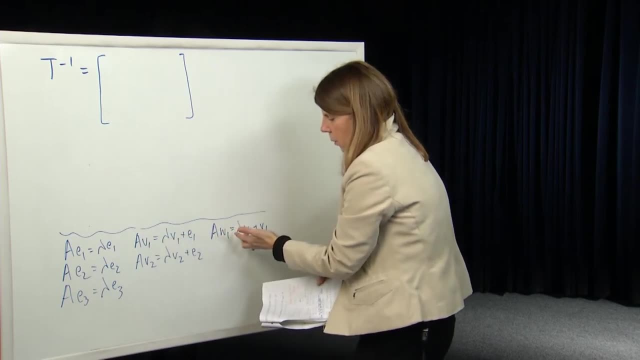 and I'm gonna write, I'm gonna order the vectors in the following way, So I can think about this row here as a chain of eigenvector: generalized eigenvector of degree one, generalized eigenvector of degree two. but they're all, they're all coming. 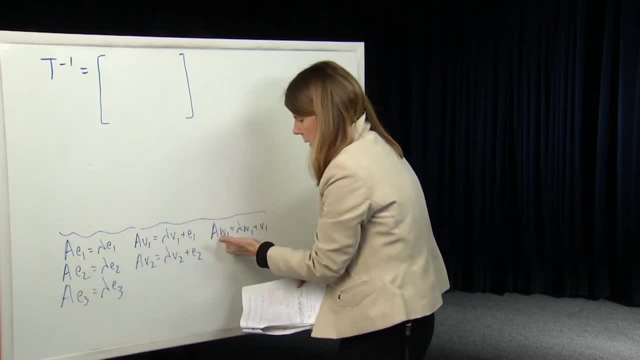 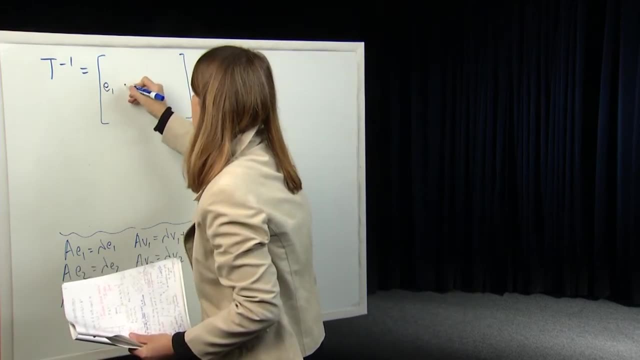 from the eigenvector E one, because V one is related to E one and W one's related to V one, which is related to E one. So I'm gonna start with my first chain of eigenvectors, generalized eigenvectors. 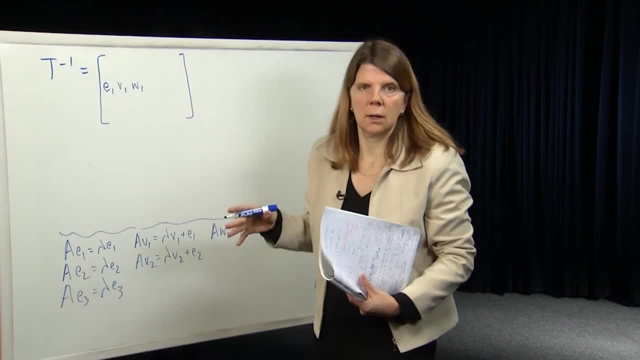 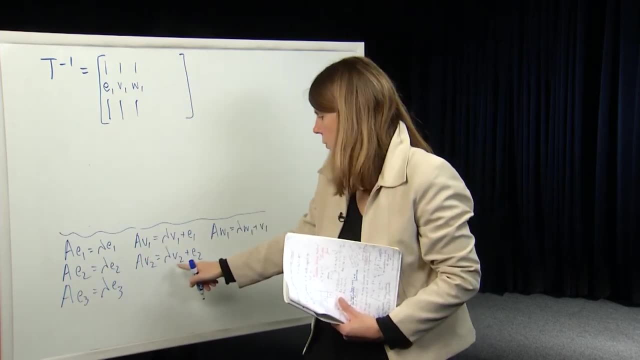 So E one, V one, W one are the first three columns of the matrix T inverse. So these are column vectors. Now I'm gonna start with my second chain. V two is related to E two, So E two, V two. 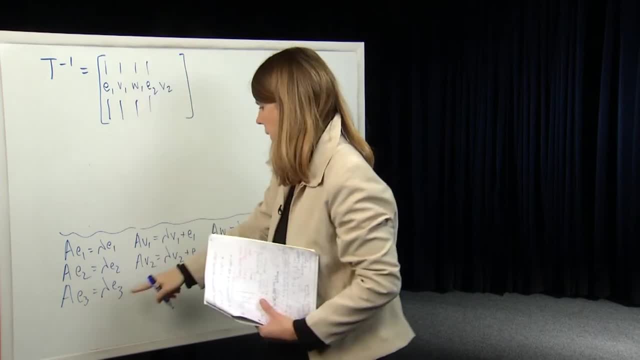 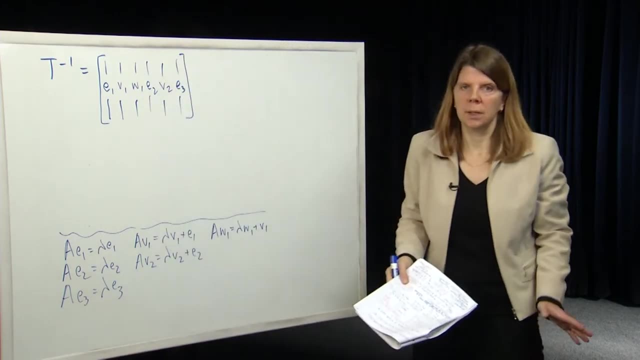 And then, finally, I'm gonna start with my second chain. V two is related to E two. And then finally, I have a last eigenvector over here, which is E three. All right, so if we construct this matrix, these are linearly independent vectors. 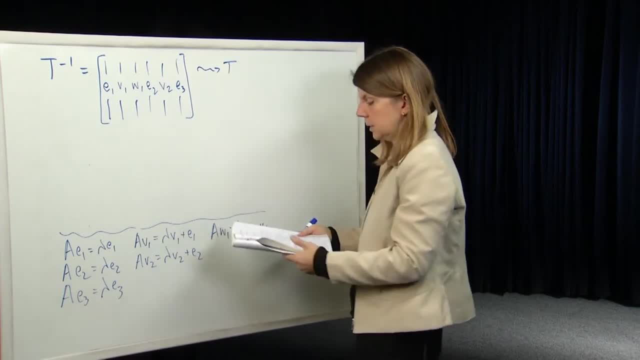 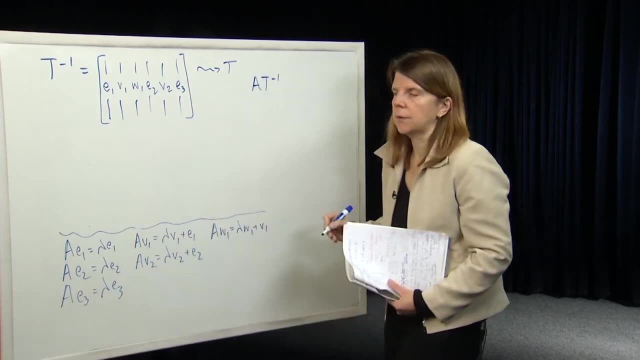 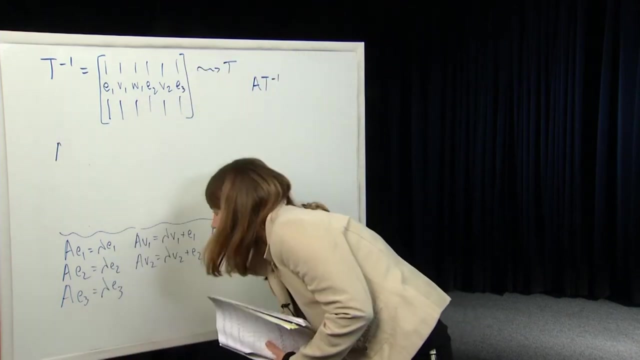 so I can compute its inverse. In particular, I can compute T Then and I go through the same thing that I did before for the diagonal case. So if I look at A T one and we can write this out, So A, so let's actually write it here. 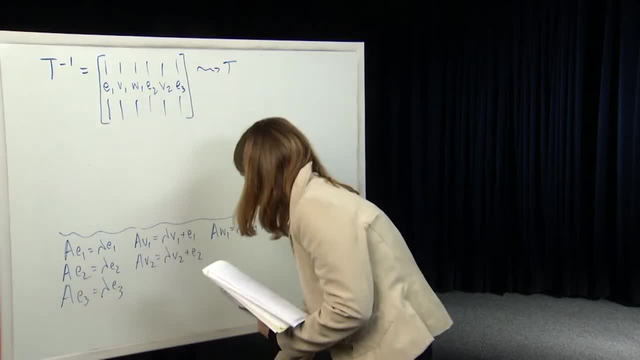 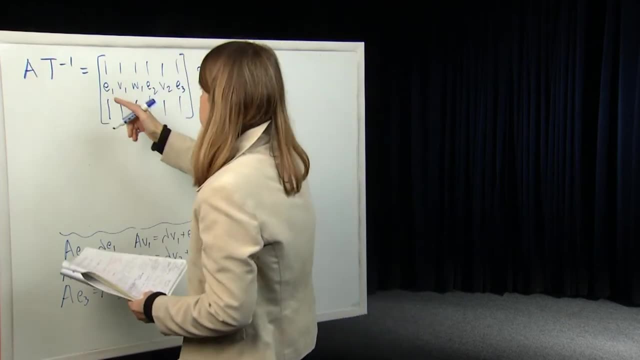 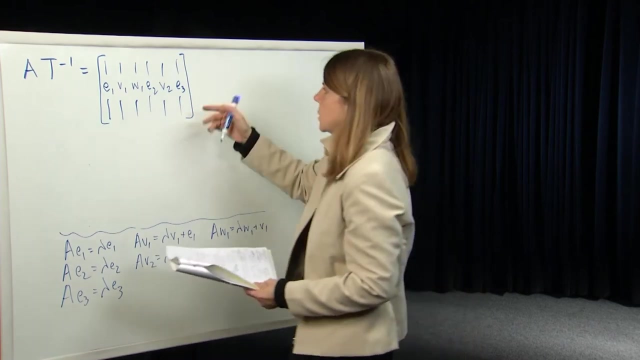 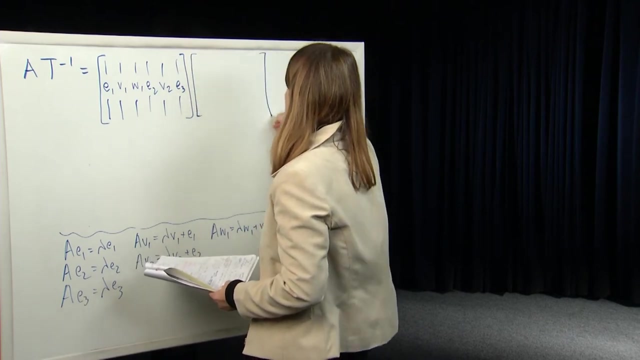 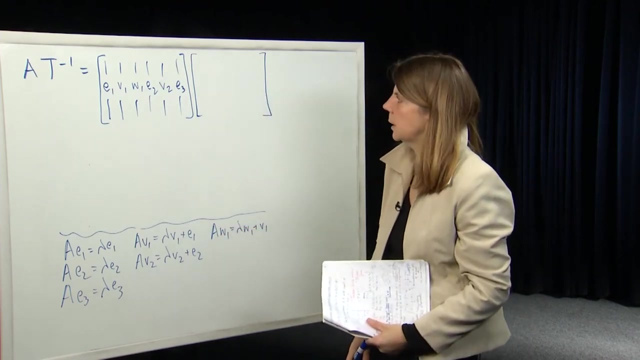 We'll use what we've already done. So A T inverse is equal to this matrix here, So it's going to be T inverse times the following matrix. Okay, so this is no longer a diagonal matrix, But from these equations we can construct what these elements are. 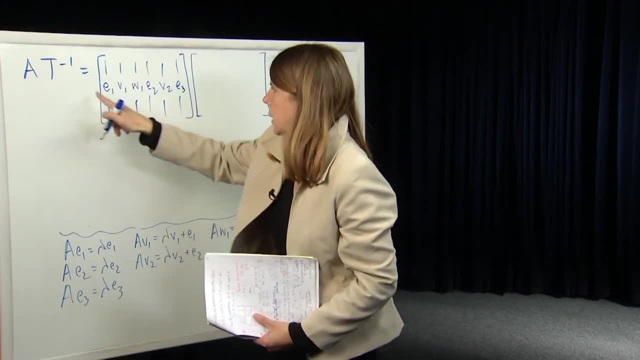 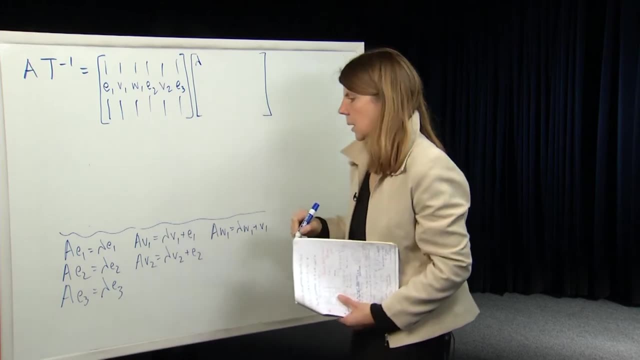 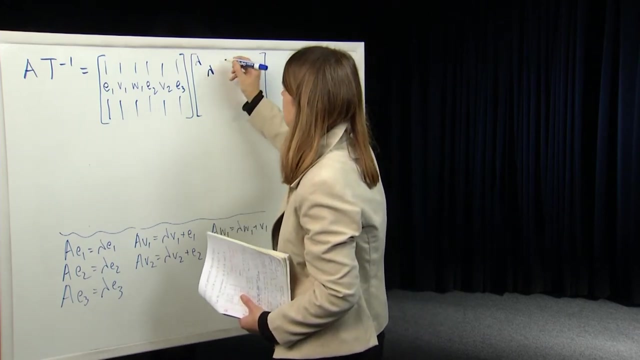 So A T inverse. so A E one is equal to lambda E one. Okay, so there's a lambda here. Now A V one is equal to lambda V one plus E one. So I have a lambda V one plus E one. 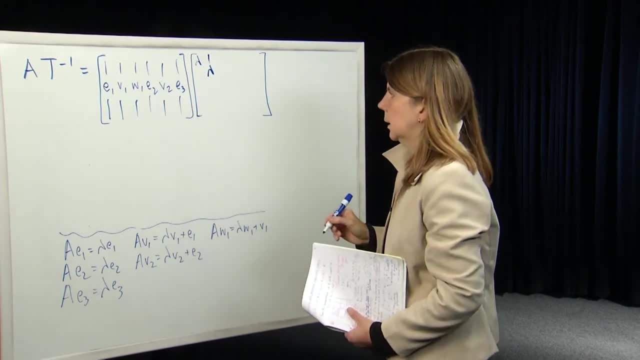 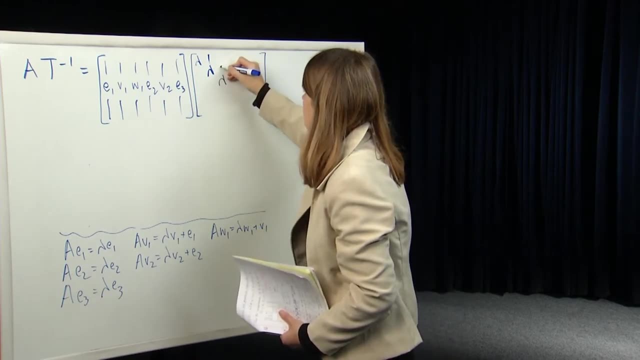 So that gives me a one up here in the super diagonal. And then what do we have? A W one equals lambda E one. A V one equals lambda W one plus V one. So a lambda on the diagonal and then a one above it. 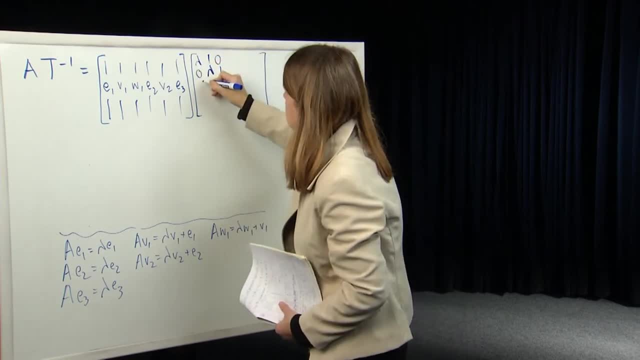 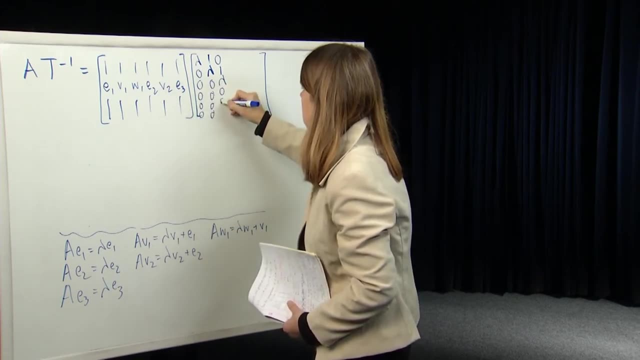 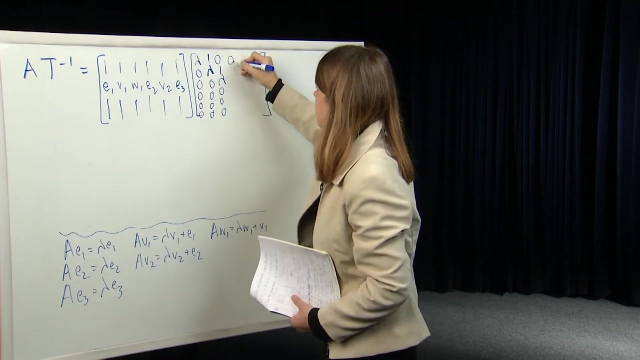 And then this up here is a zero, And then everything else here is zeros: Four, five, six, All right, so that's the first three columns, And now we go to the second row. A E two is equal to lambda E two. 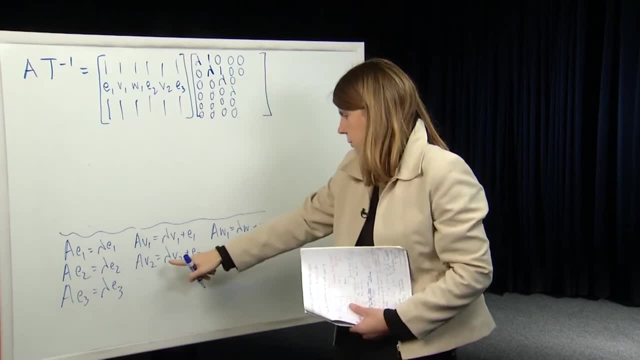 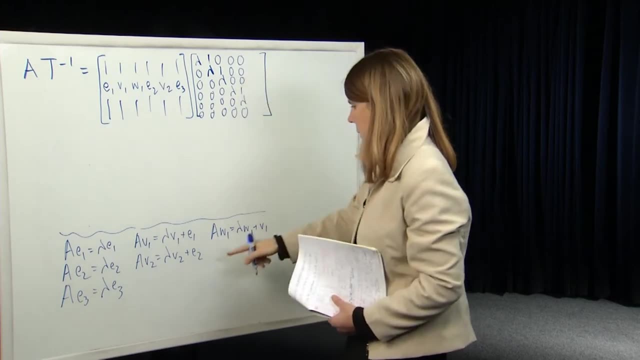 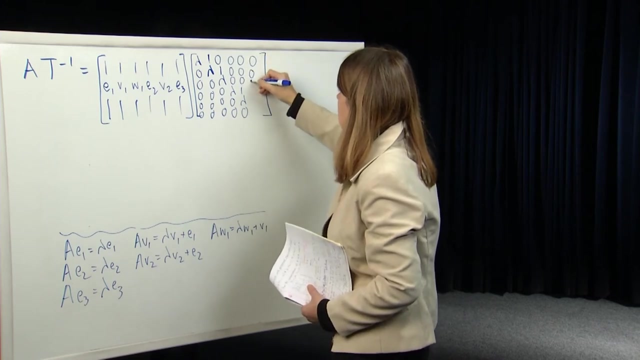 A V two, A V two, A V two is equal to lambda V two plus E two, So it's a lambda one like that. And then finally A W one is lambda W one. sorry, A E three is equal to lambda E three. 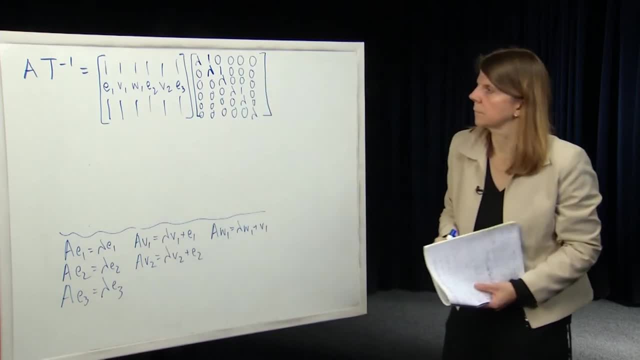 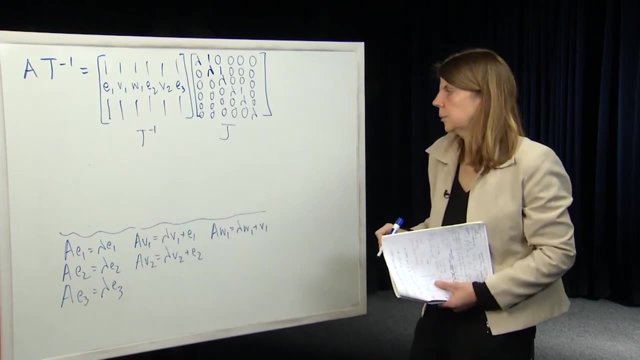 So that's just a lambda here. Okay, so A T inverse is equal to T inverse J, where J is called the Jordan form of the matrix A And in general now we can write post-module matrix A. it's called the Jordan form of the matrix A And in general now we can write post-modular matrix A. 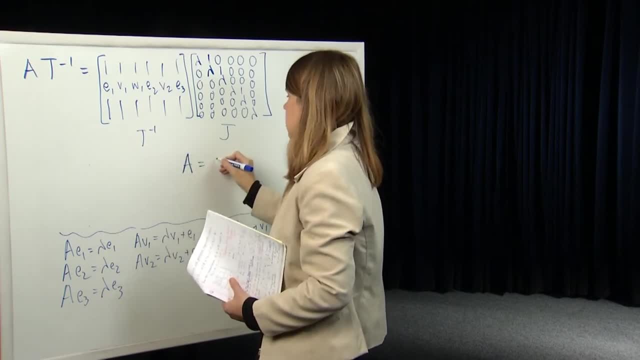 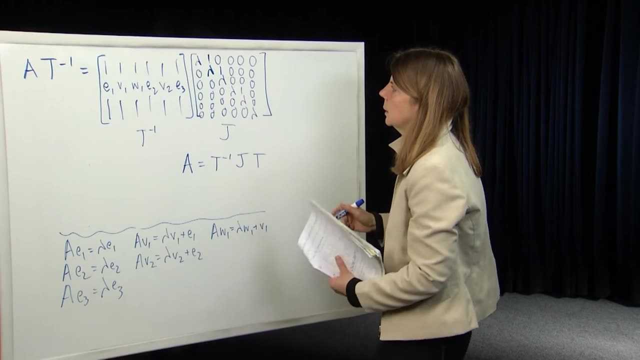 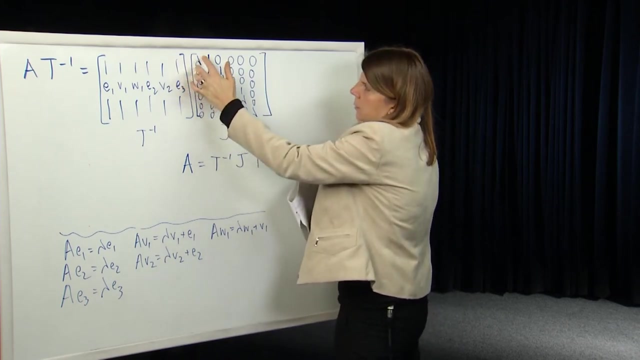 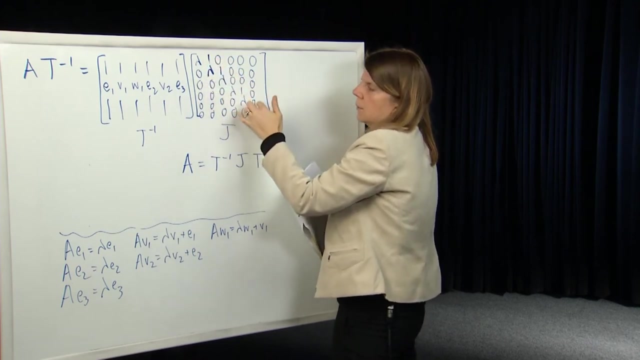 post. multiply by t here, so a is equal to t, inverse j, t, where j has this following form: so let's take a look at it. we have- it's a upper triangular matrix where we have, where we have the eigenvalue lambda on the diagonals and on the super diagonals we have 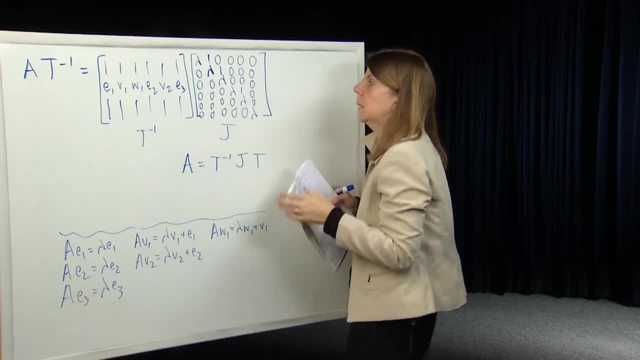 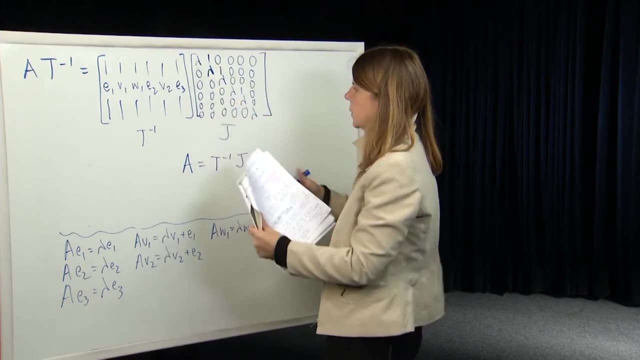 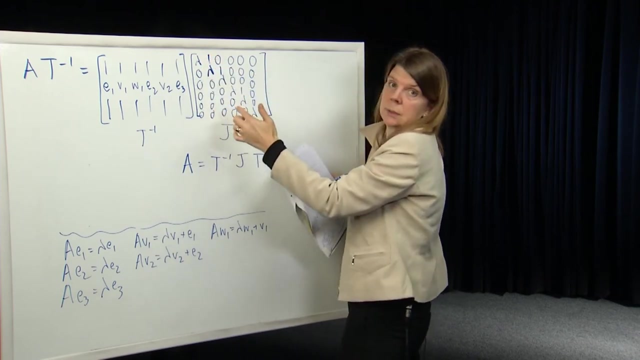 either ones or zeros, and then everything else is zero, okay and associated, so associated to the lambda. so depending on whether or not we have a eigenvector, so you can see that all the columns that are associated to eigenvectors are all zeros, but columns associated to generalized eigenvectors. 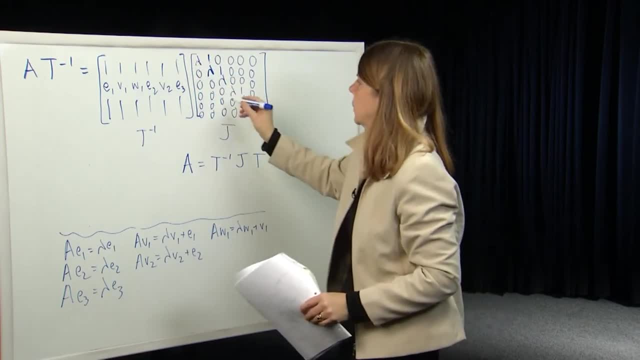 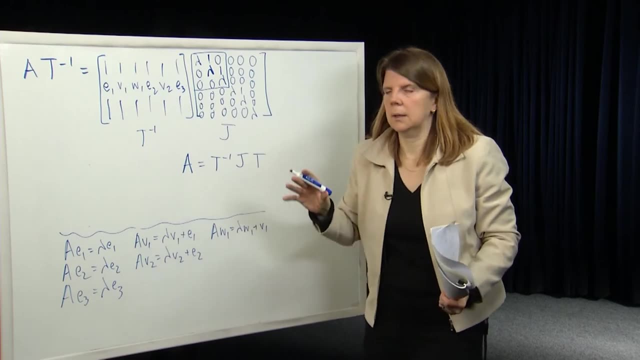 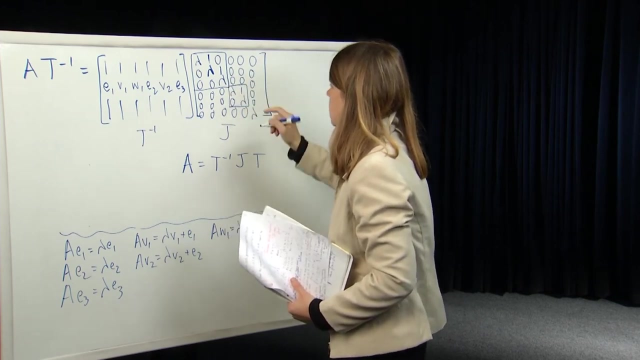 have a one on the super diagonal and from this we can derive what we mean by jordan blocks. so i can represent this matrix as a diagonal at a matrix whose diagonals are blocks or, sorry, as a matrix who has diagonal block matrix entries, or it who has block matrix. 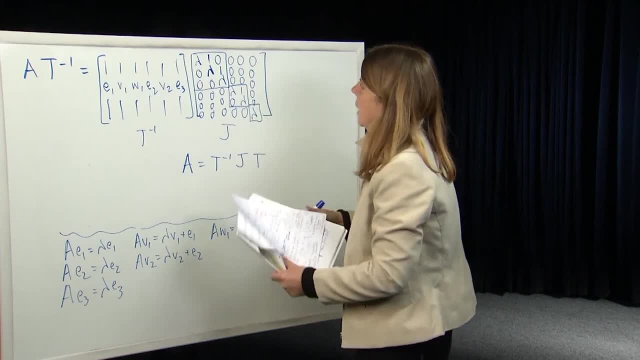 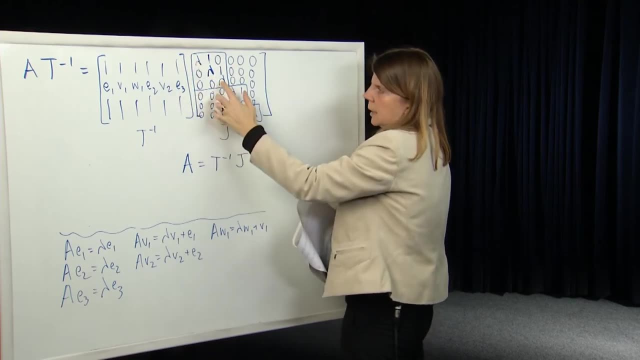 entries on the diagonal and in this case i have a block and then everything else is zero. so i have a block which is a three by three block associated to the eigenvalue of lambda, a two by two block and a one by one block. so this is called a Jordan block of size two. 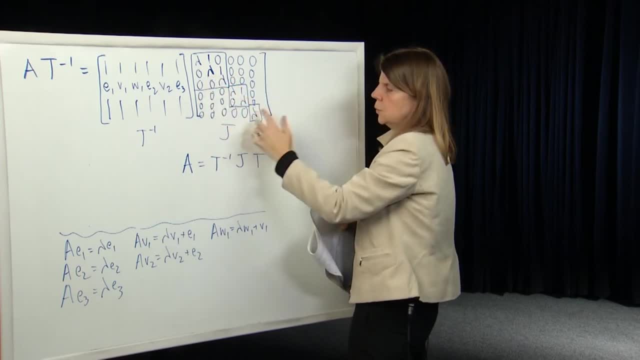 of the eigenvalue lambda, and also known as desaline, called a jordan block of size two of two… or sorry, a Jordan block of size 3,, a Jordan block of size 2, and a Jordan block of size 1.. 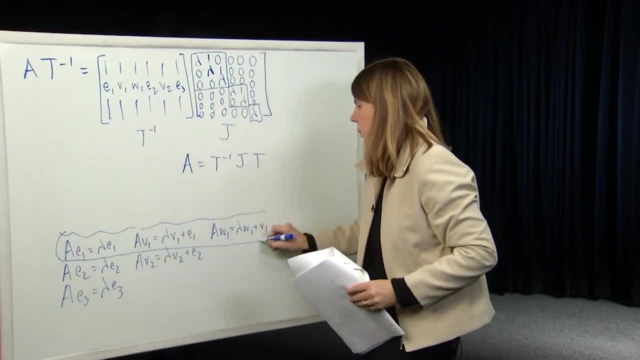 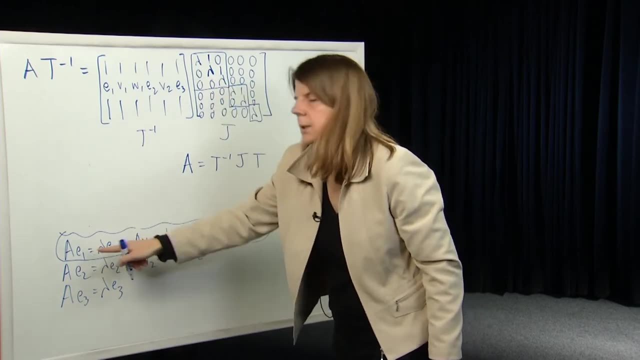 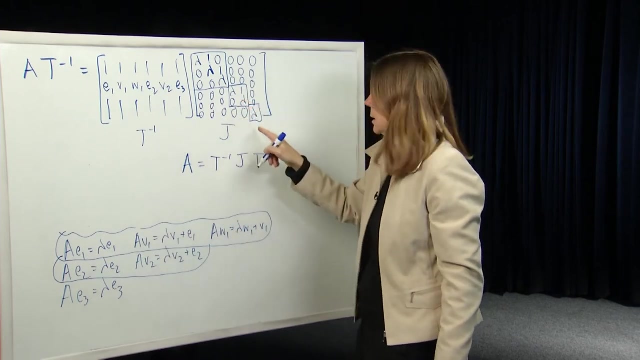 And that Jordan block of size 3 came from the fact that there was one eigenvector and two generalized eigenvectors associated to lambda, when the eigenvector is E1. There is one eigenvector and one generalized eigenvector associated to E2, and one eigenvector associated to E3. There's no. 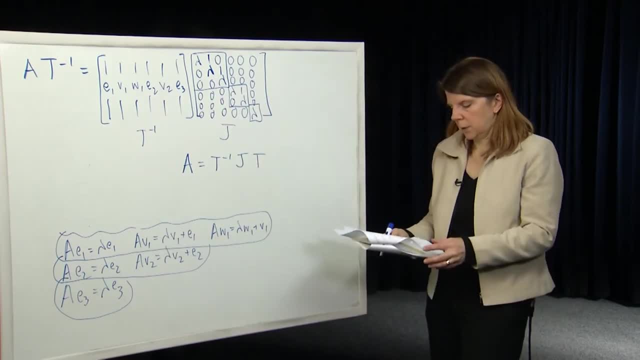 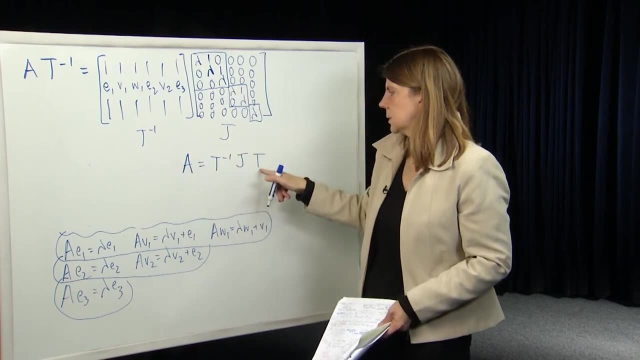 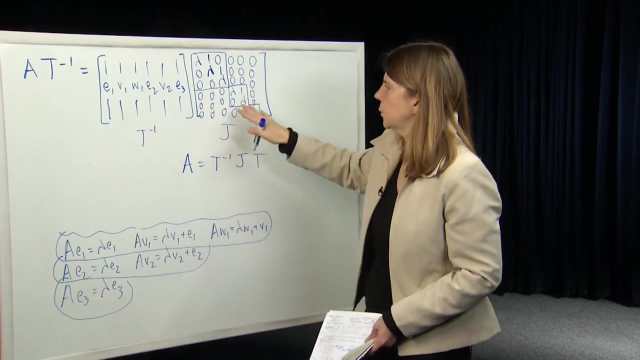 generalized eigenvectors. Okay, so that's an example where we constructed the similarity transform. So this matrix T, inverse, it's invertible, And this says that for any n by n matrix A, you can construct a Jordan form by constructing eigenvectors. And then really, 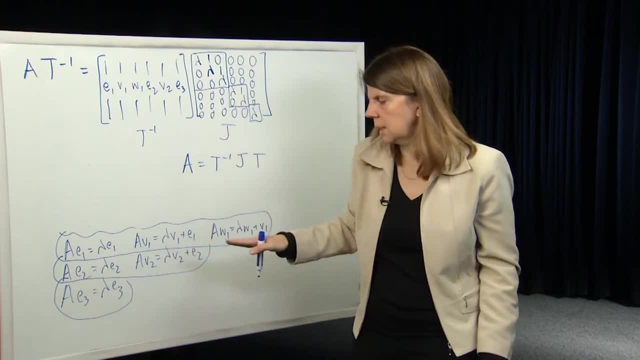 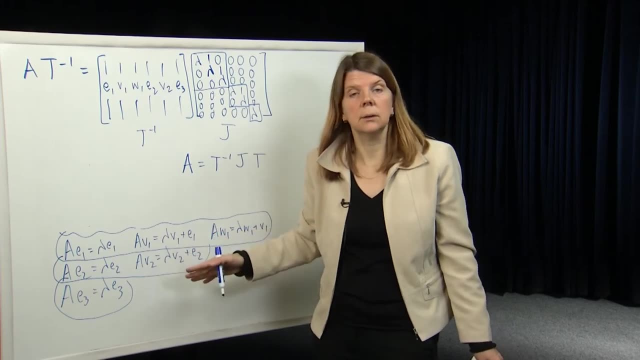 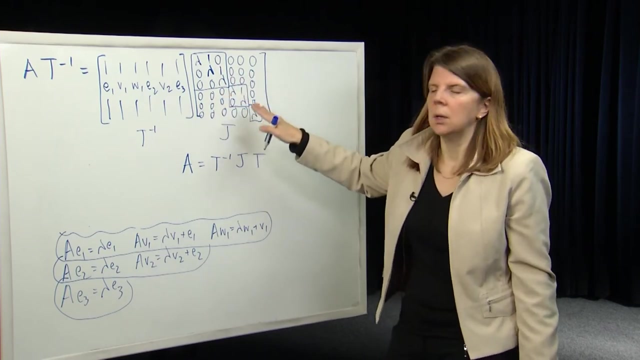 these are just mathematical entities that we define as generalized eigenvectors. The point is that you can always define n, or in this case six linearly independent vectors, which gives you a similarity transform of A to the following form, which, for the non-diagonalizable matrices, is as simple as you can get: Okay. 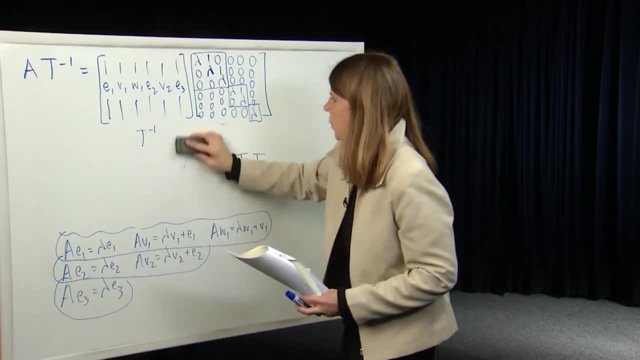 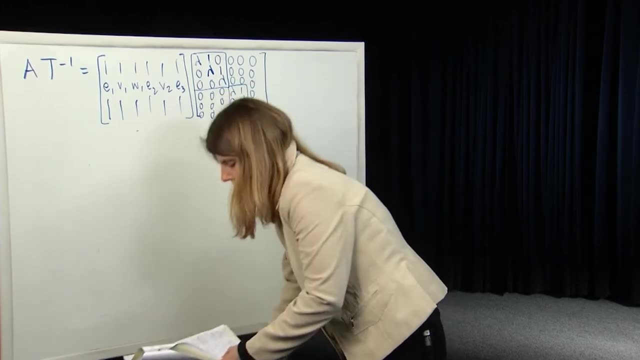 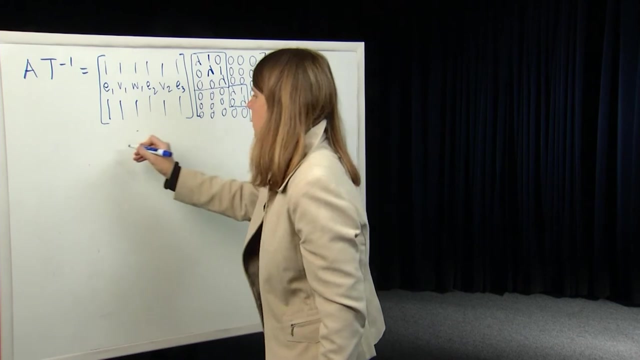 so we have that Jordan form. for our case where we had a six by six matrix with basically six repeated eigenvalues at lambda, What would happen if you had, you know, a general Jordan form You might have. so in general, you could have a Jordan form. 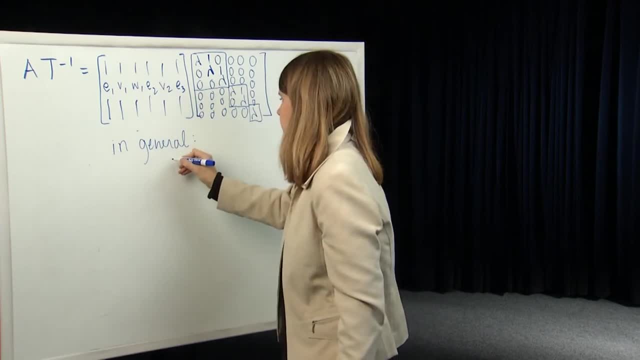 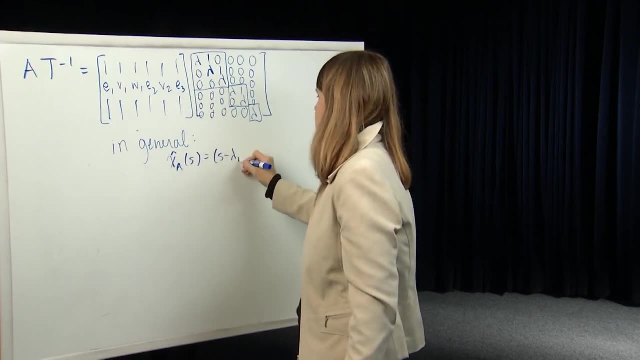 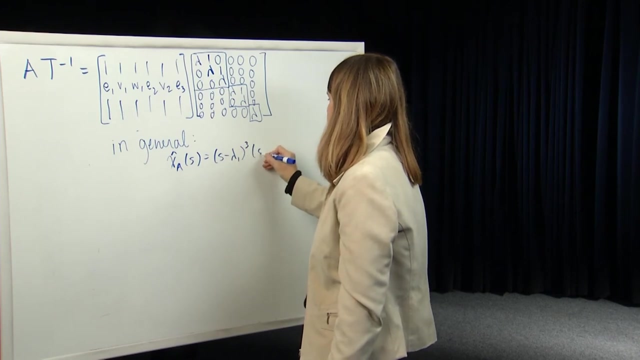 that looks like. suppose you had a characteristic polynomial which was of s, which is s minus lambda one. Let's just suppose we have two eigenvalues and we can generalize this to n, And that was three, and s minus lambda two, which was of dimension two. So this is a five. 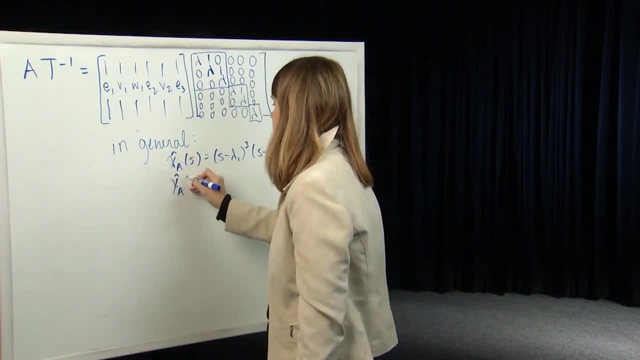 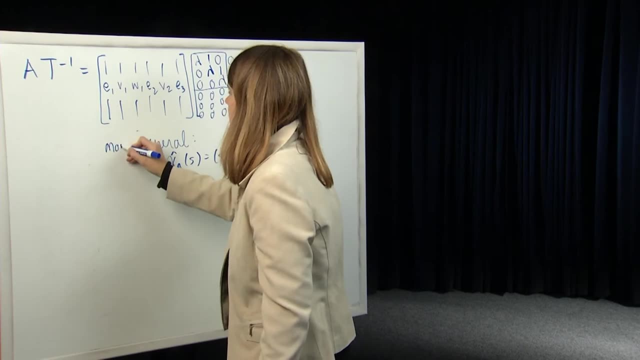 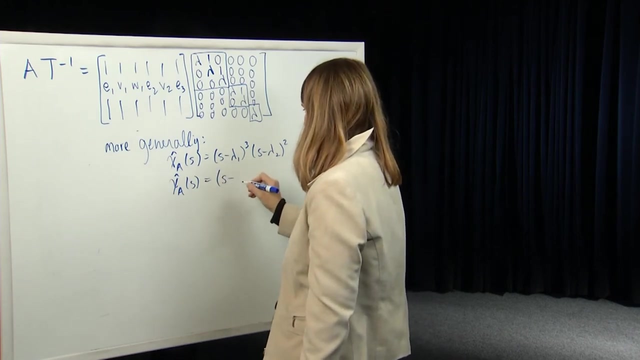 by five. matrix A: Let's suppose that the minimum polynomial. so I shouldn't really say in general, but more generally, let's say- because we're still looking at a specific example- more generally. But now I've expanded to two eigenvalues And so let's get this one. 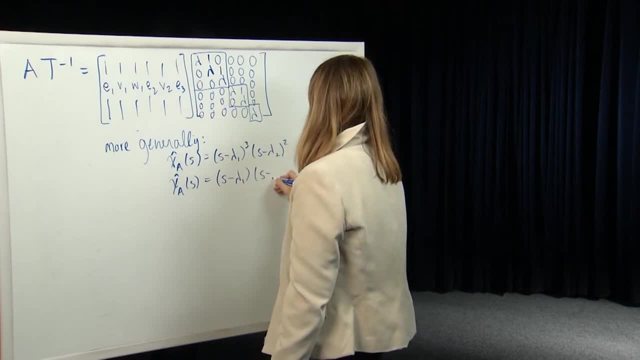 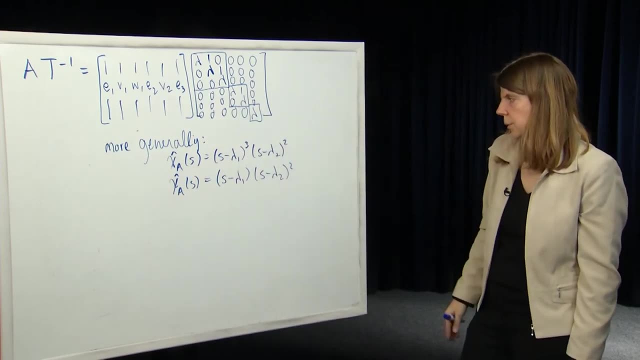 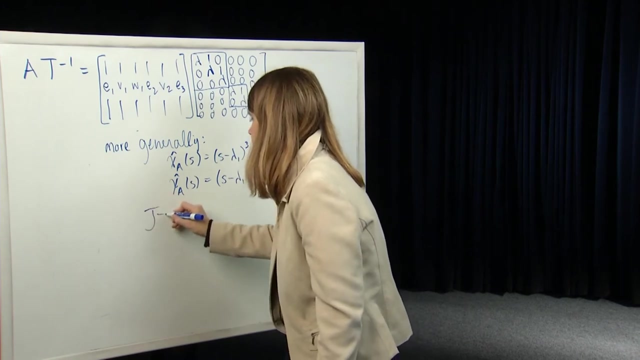 Let's suppose it's just s minus lambda one, And let's make this one s minus lambda two squared. Okay, so the minimum polynomial is as of degree three in this characteristic polynomial of degree five. So just from that information now you can construct possibilities. 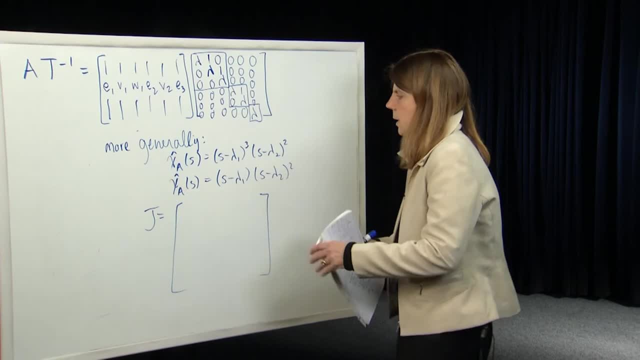 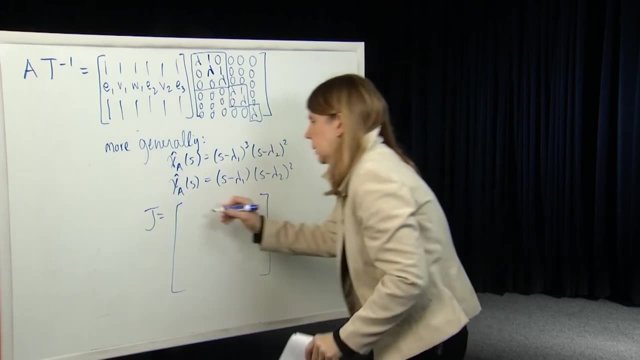 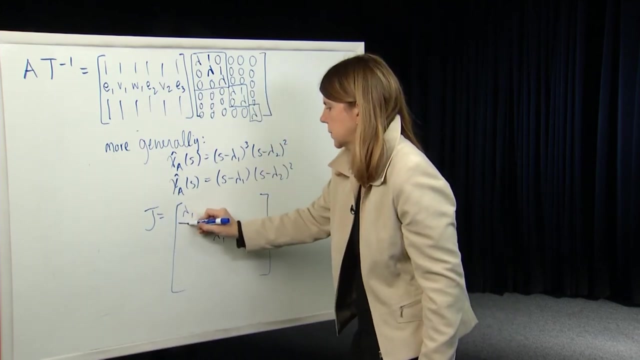 of what the Jordan form looks like. So what this says is that the largest Jordan block associated to eigenvalue at lambda one is of size one. So that tells you that the Jordan form for each of those, the largest Jordan block, is of size one. 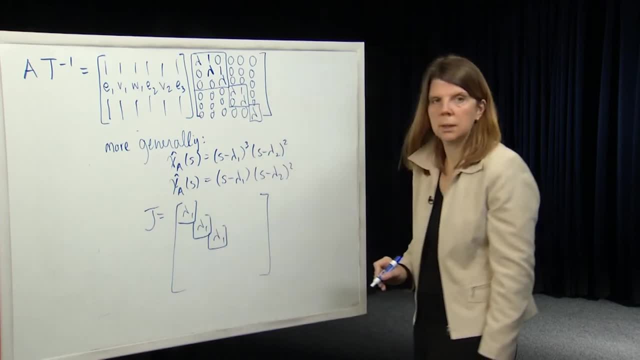 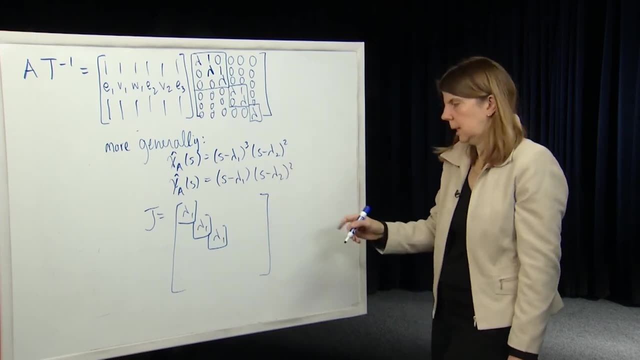 so I'm gonna get three little blocks of size one associated to the eigenvalue at lambda one, And then the Jordan block. the largest Jordan block associated to the eigenvalue at lambda two is two, so that should be lambda two. so that tells you. 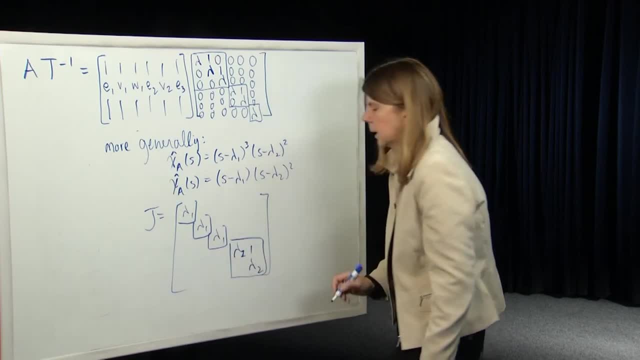 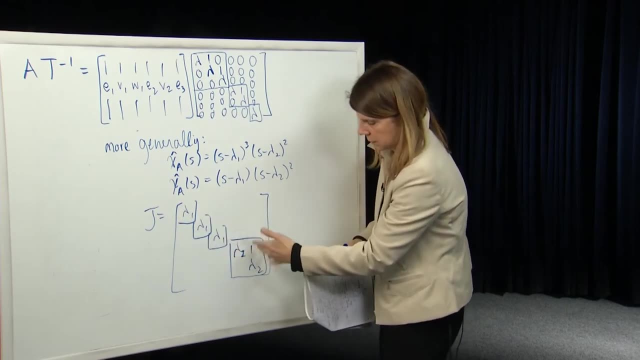 that the Jordan form is gonna look like this. Now we say the Jordan form will look like that. that's up to permutation. so I could've reordered the eigenvectors and generalized eigenvectors in this case, so I might have this block appearing here. 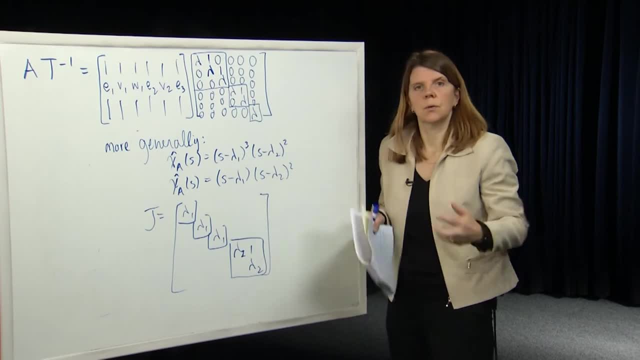 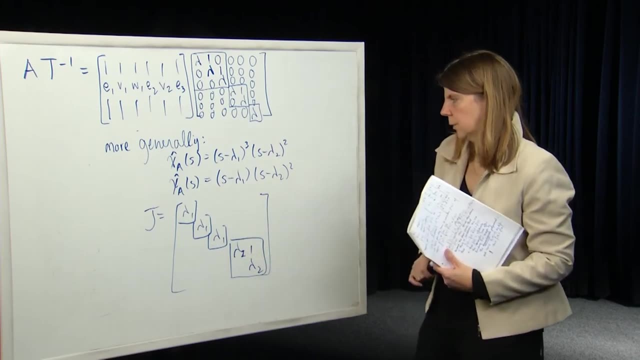 and these smaller blocks appearing here, We consider that the same Jordan form up to permutations of the Jordan block. Okay, so in this case this gives us only one possibility for the Jordan block. Let's see. could I have had other possibilities? 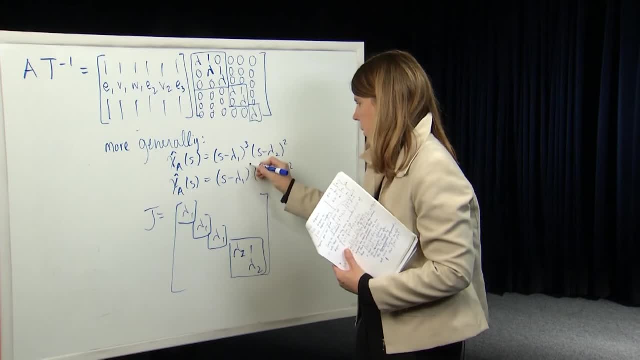 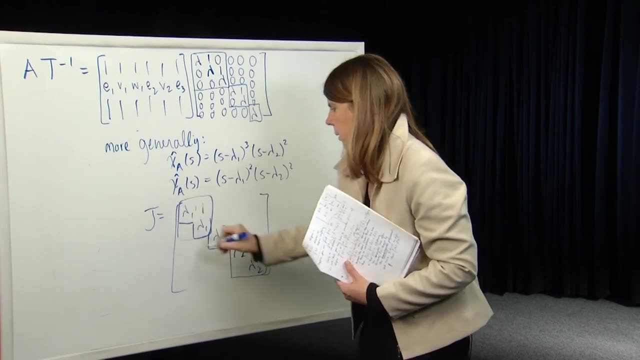 Three. no, because if I had two here, two, that would've specified that I would've had a Jordan block of size two and a Jordan block of size one. That's the only way to get that here, But in different cases, if you're given. 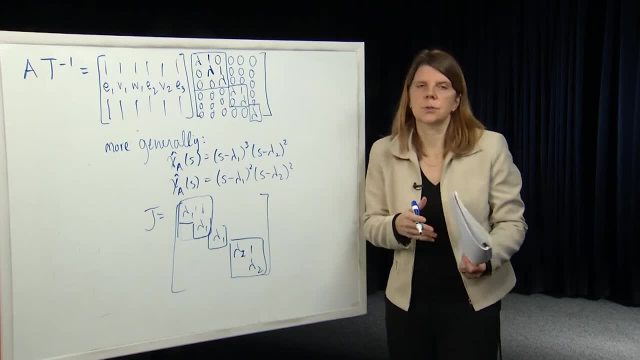 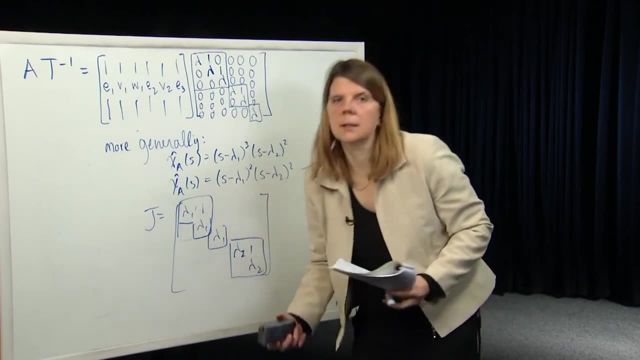 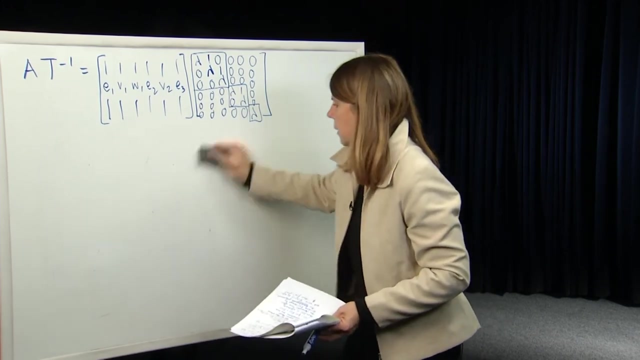 the characteristic polynomial and the minimum polynomial, you can come up with constraints on what the Jordan form looks like. All right. finally, let's conclude with why this is useful In the diagonal case. the whole point was: it's useful because you can come up with a formulation. 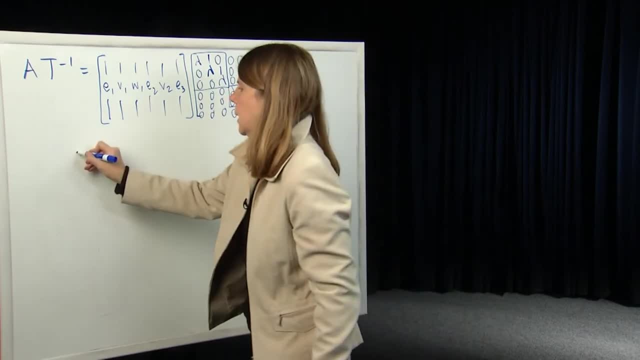 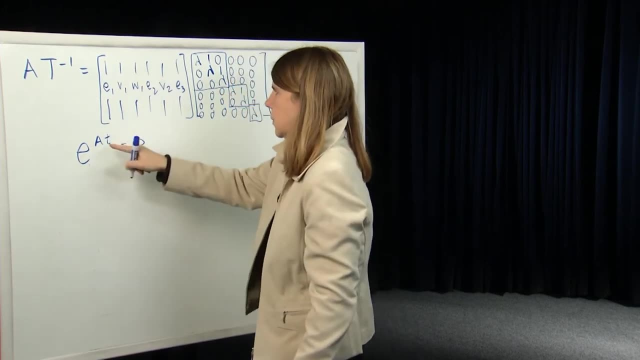 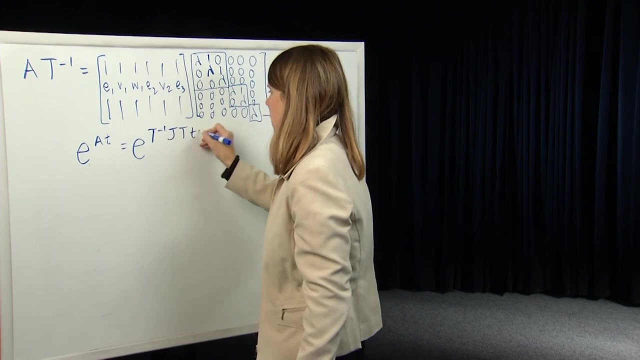 of e to the at more easily. So we remember that e to the at is equal to e to the in this case. now it's gonna be so: a is t inverse jt, which we showed before. is t inverse e to the jt- t. 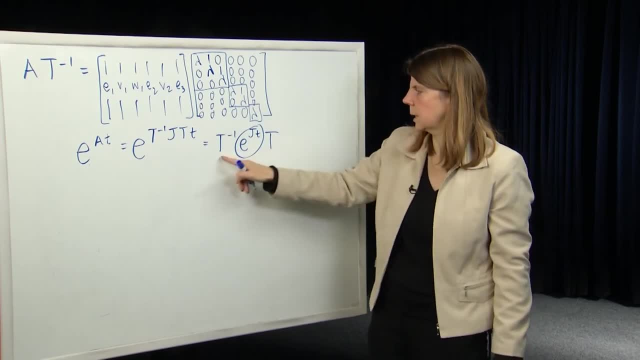 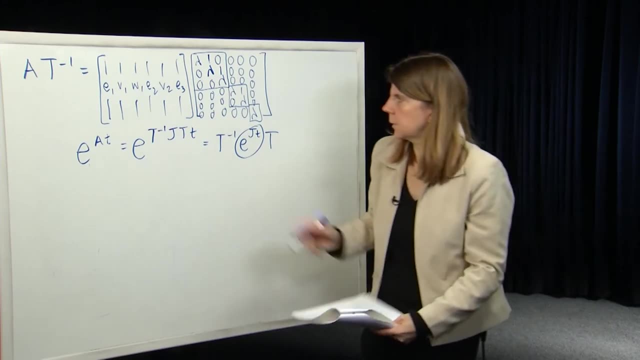 So it's really this that we're interested in computing: because we can always get back and forth to e, to the at, by pre- and post-multiplying by these n by n invertible matrices. Okay, so we have then a general result which tells us: 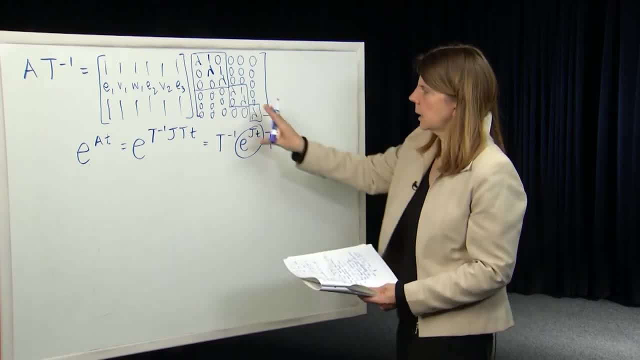 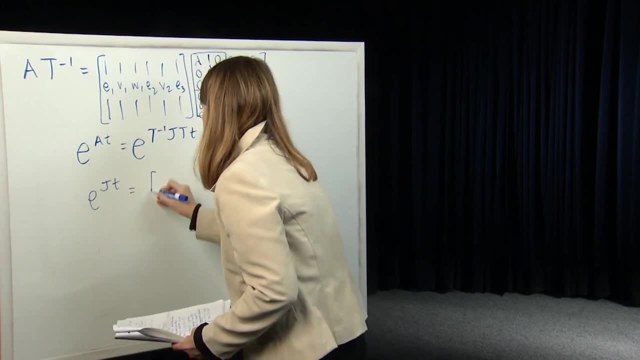 Okay, so we have, then, a general result. Okay, so we have, then, a general result which tells us so, just like we had for the diagonal form, for the Jordan form, if the general Jordan form, well, let's just use the example that we have above. 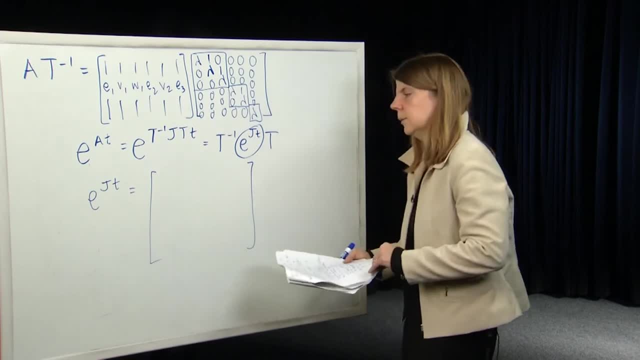 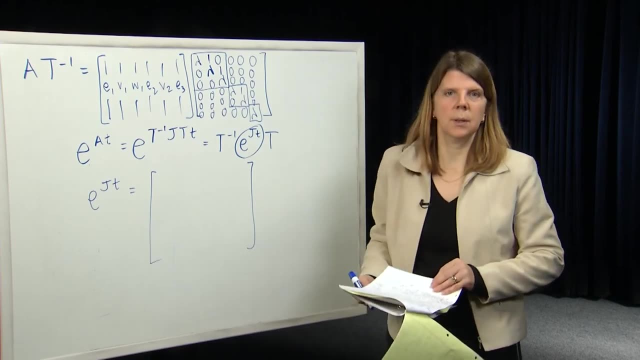 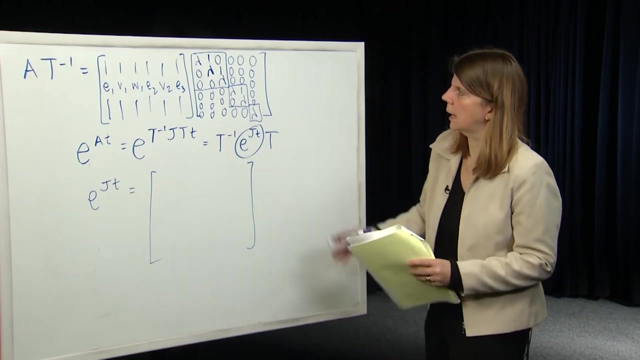 looks as follows: then e to the jt. well, we can do a more general example as well, but e to the jt will have quite a specific form and it can be computed just by inspection. So, just like in the case where we had the diagonal form, 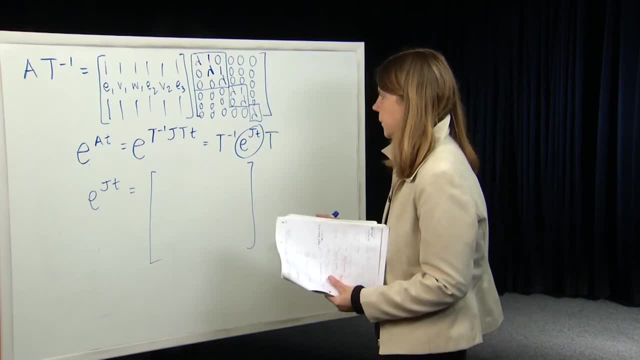 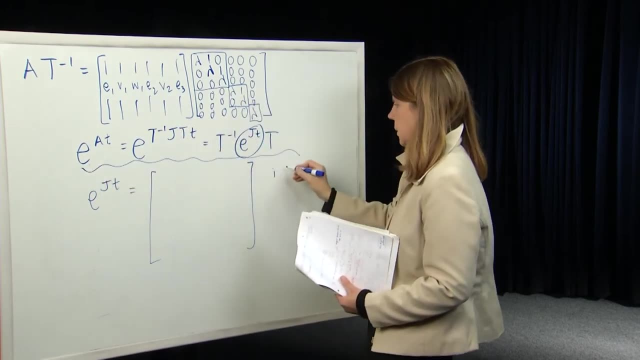 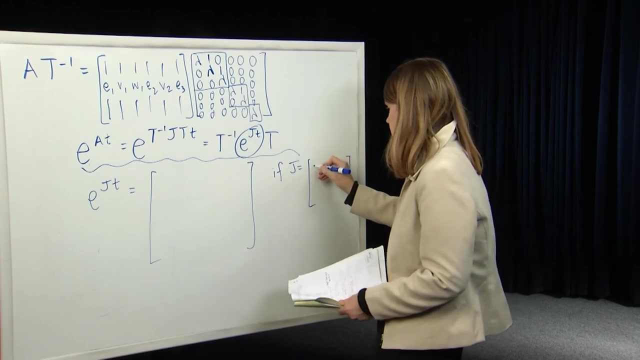 and we could do it by inspection, if this is, let's actually do a couple of cases. so if we'll separate ourselves from this example here, suppose we had a Jordan matrix that just looked like one Jordan block, so lambda's on the diagonal and one's on the superdiagonal. 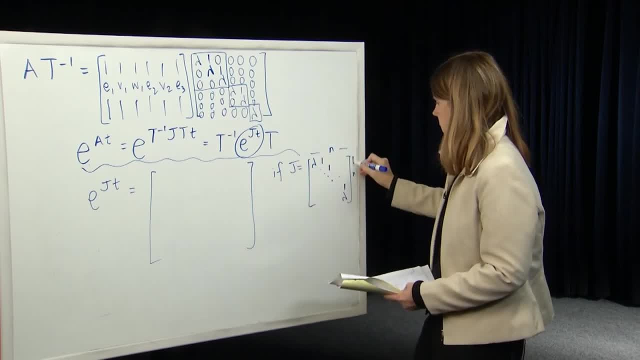 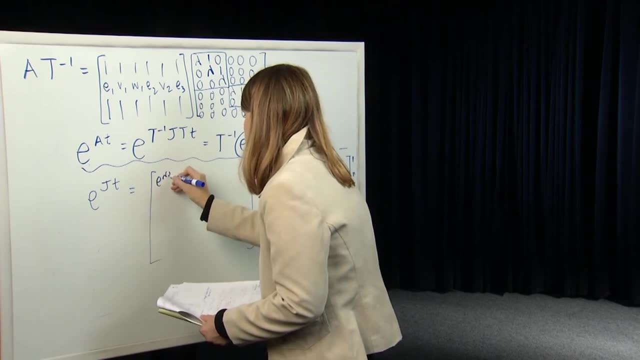 So that's a Jordan block of size n, then f of j or e to the jt and then e to the jt, where e to the jt is going to look like e to the lambda t on the diagonals, just like in the diagonal case. 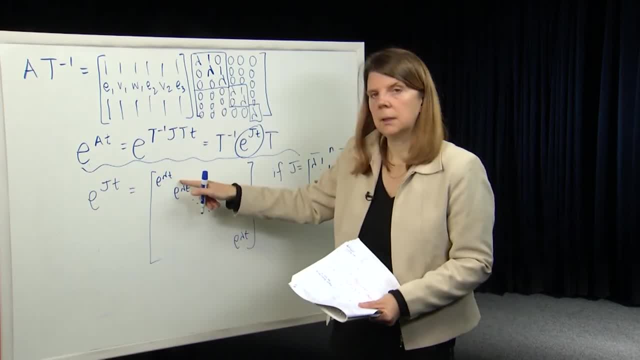 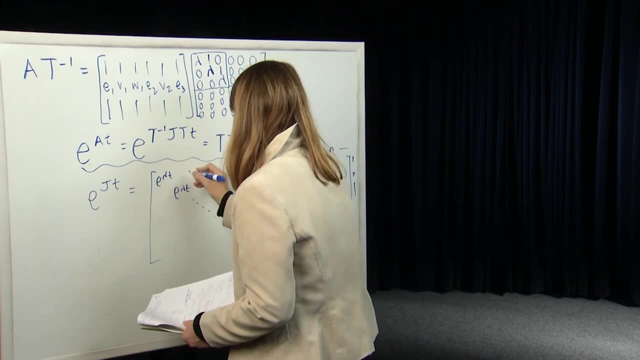 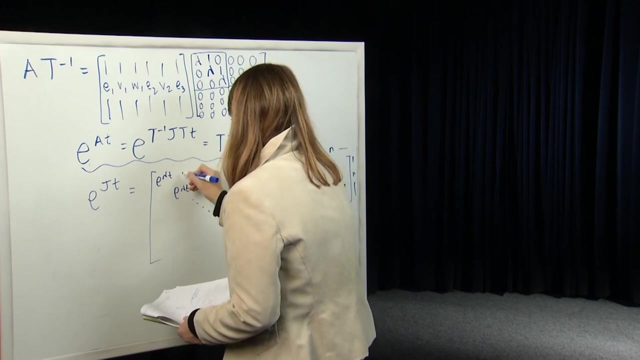 So the eigenvalues of e to the jt are e to the lambda t, where lambda is the eigenvalue of j, And then on the superdiagonal we'll have the derivative of e to the jt. So that's lambda, or let's just call it. 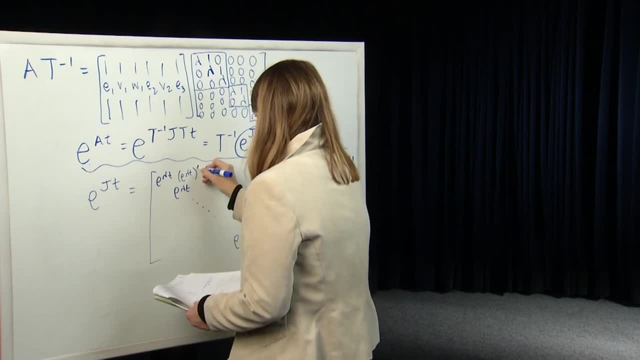 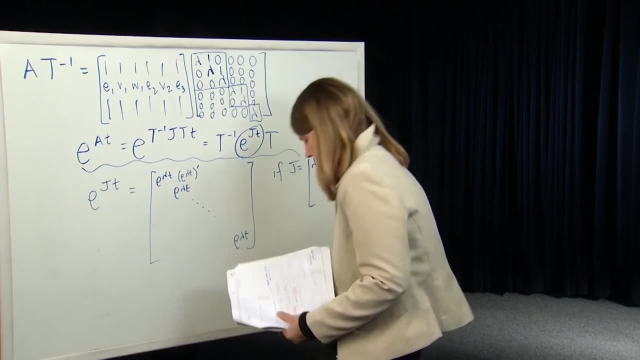 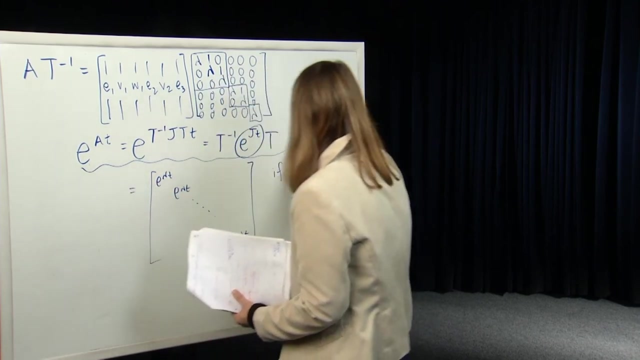 e to the lambda, t derivative with respect to t, So d by dt of e to the lambda- No, sorry, e to the. this is with respect to lambda. Actually, let's be a little more general. Let's suppose we had this matrix j. 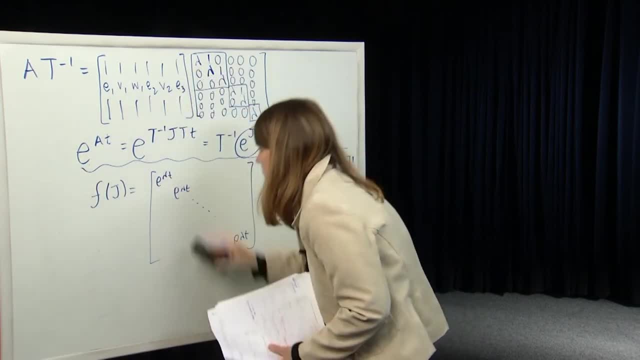 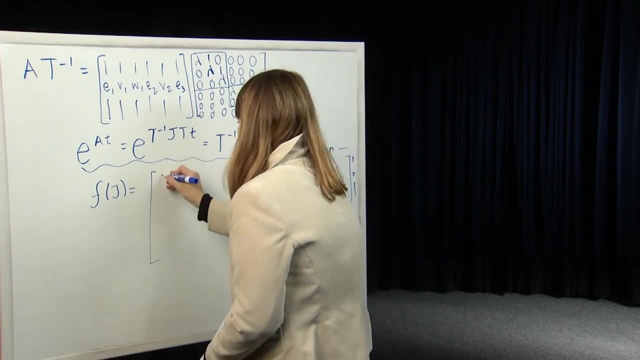 and we were computing a function of the matrix j. So we can generalize or we can make this specific to e, to the lambda t, in a second. Then what does f of j and what does the f function of j look like? This is f of lambda on the diagonals. 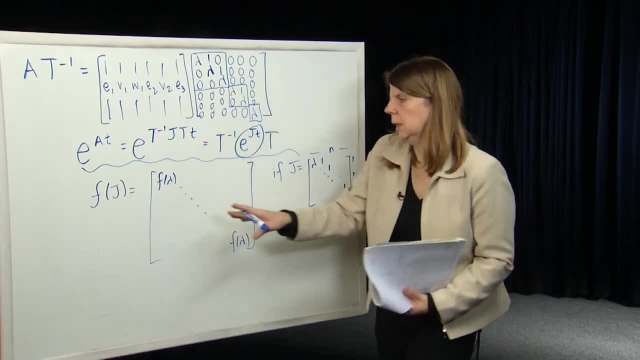 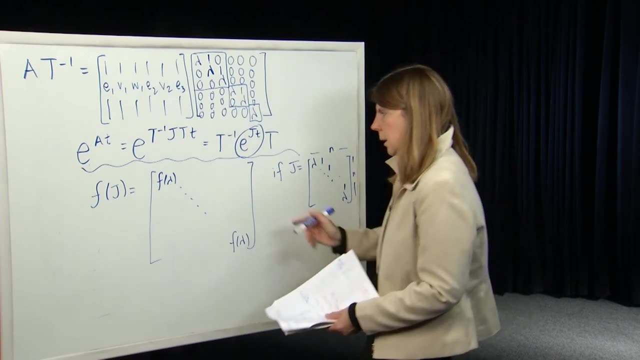 Okay, so this is a function. in our case it's e to the jt, but in general this result holds for any function f which is analytic on the domain, on the spectrum of a And what we have on the superdiagonal. 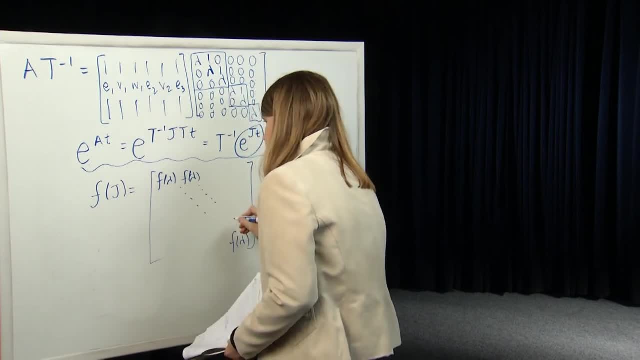 is the derivative of f with respect to its independent variable, so s or whatever, and then evaluated at lambda. And then on the super superdiagonal f dot farbeit, let's write that down. We think that's F for lambda, four times aph harmful to lambda. 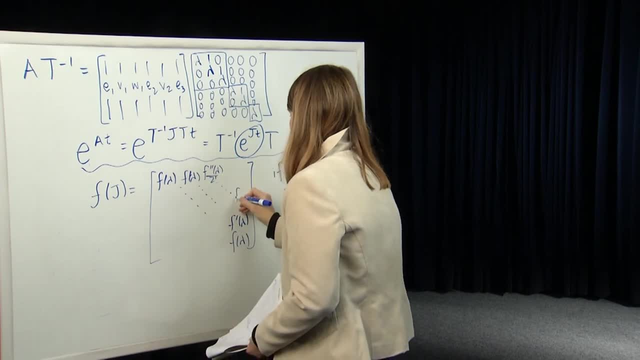 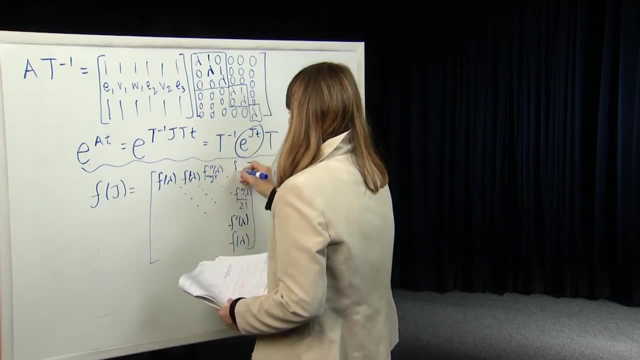 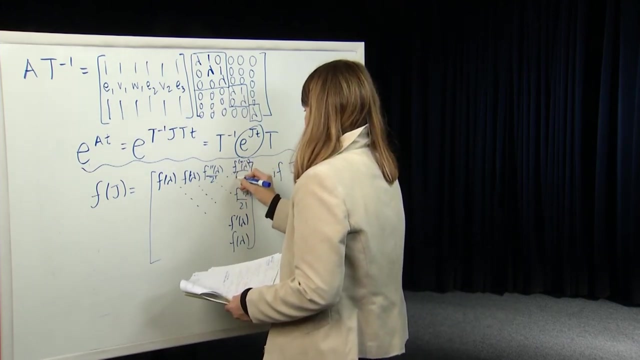 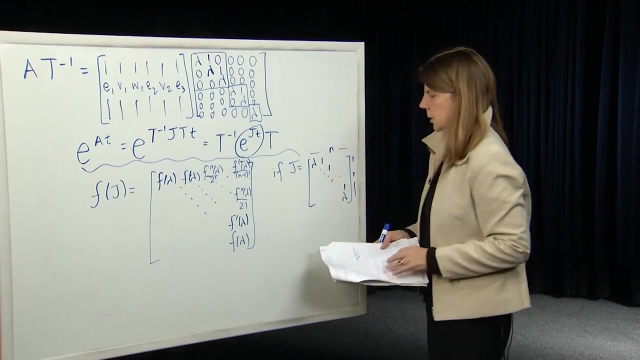 double prime of lambda over two factorial. f double prime of lambda over two factorial. all the way up to the top right corner element, which is the n minus first derivative of this function: f evaluated at lambda over n minus one factorial. So that's the general form of a function, of a matrix. 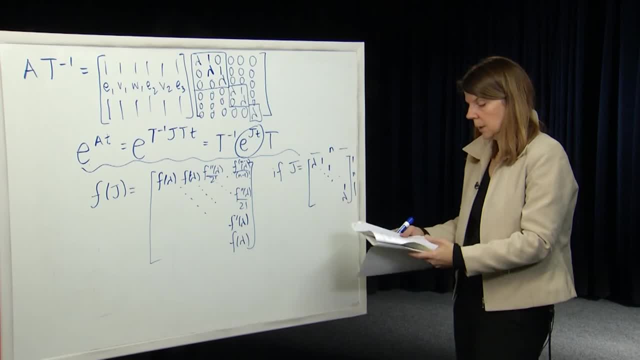 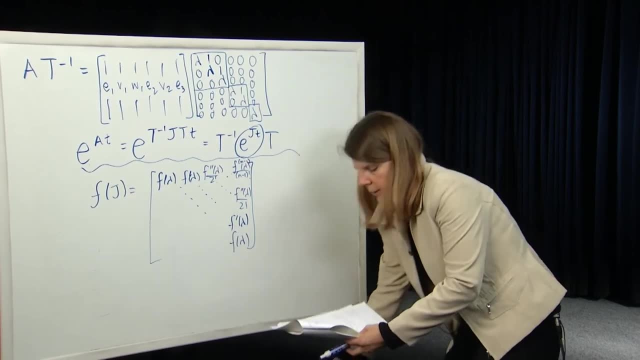 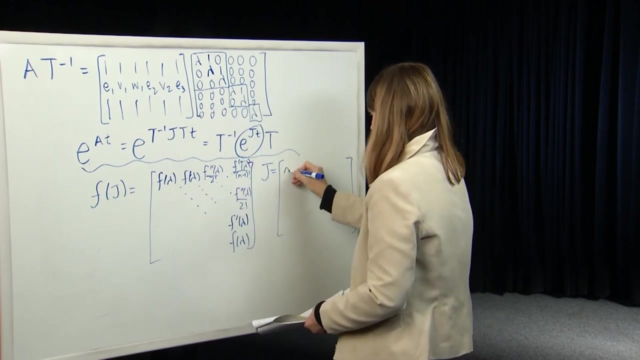 if the matrix is in Jordan form and if we had a more general form. so suppose now our J looks like it has several Jordan blocks. Okay, so let's just do an example similar to the one we had before. So let's suppose I have three eigenvalues at lambda one. 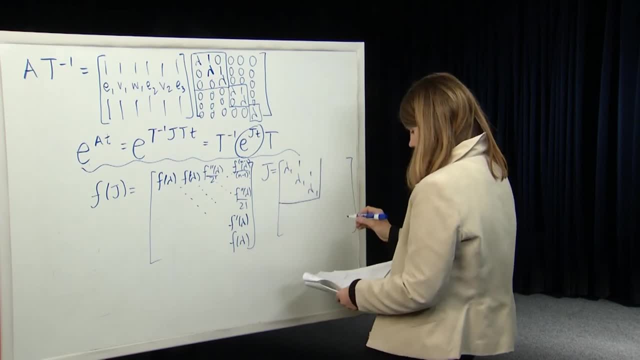 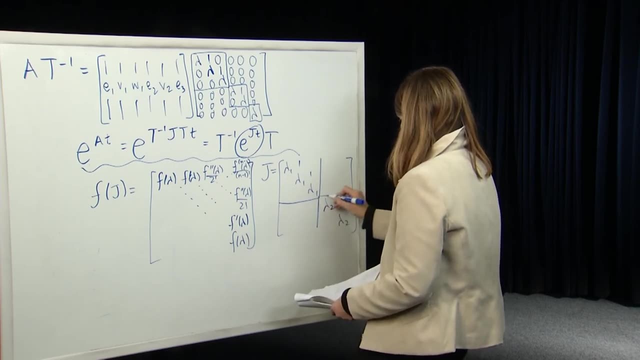 Actually we've got a Jordan block of size three here. Let's put a Jordan form, let's put two eigenvalues at lambda two and let's put a two by two Jordan form there. Then you can just take this result for f of J. 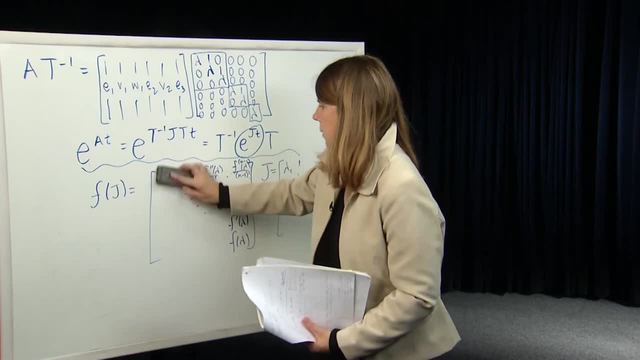 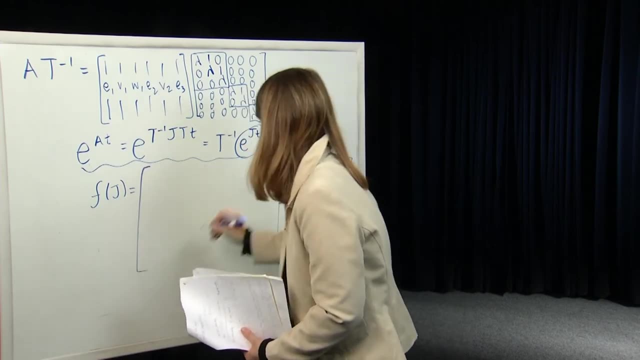 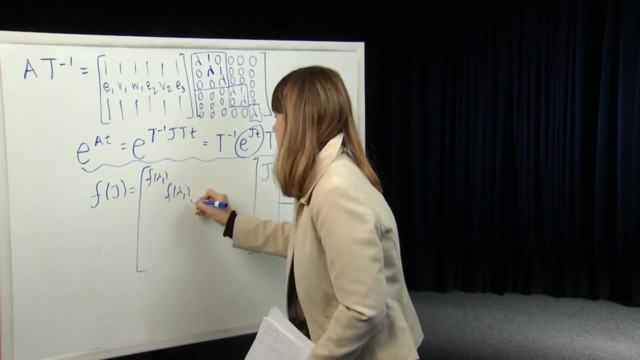 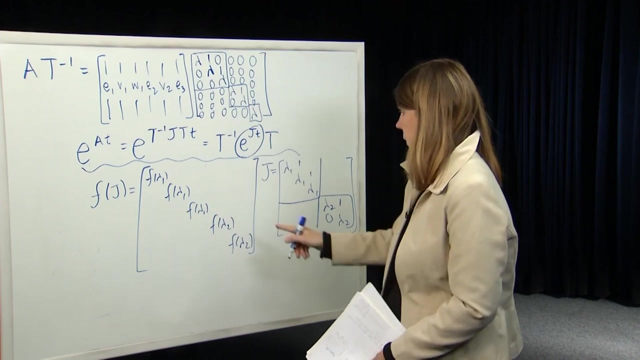 and extrapolate it, and extrapolate it. So here f of J is. so we have f of lambda, one f of lambda, one f of lambda, one f of lambda, two f of lambda, two on the diagonal and then on the super diagonal. 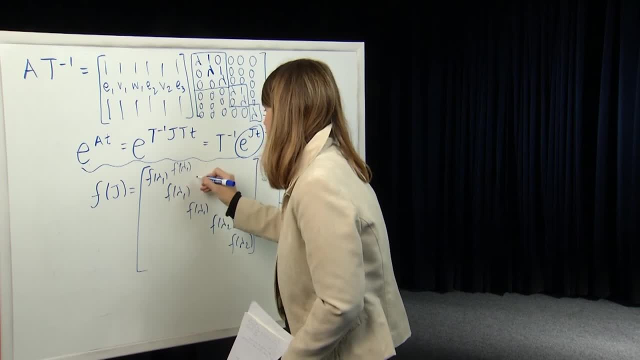 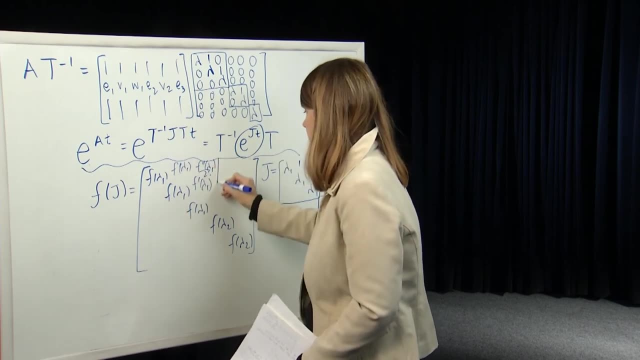 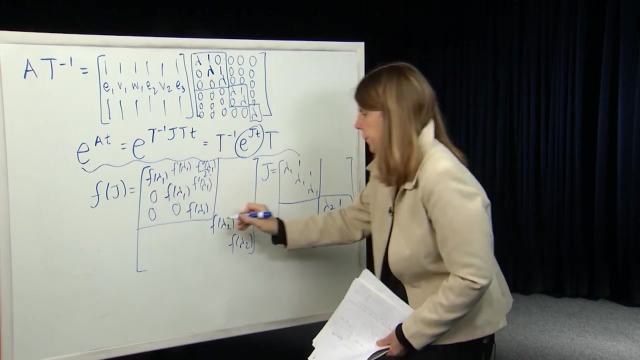 we're going to have f prime of lambda one, f prime of lambda one, and then f double prime of lambda one over two factorial up in the corner there. Okay, so there's a three by three block and the rest are zeros. that comes from this Jordan block. 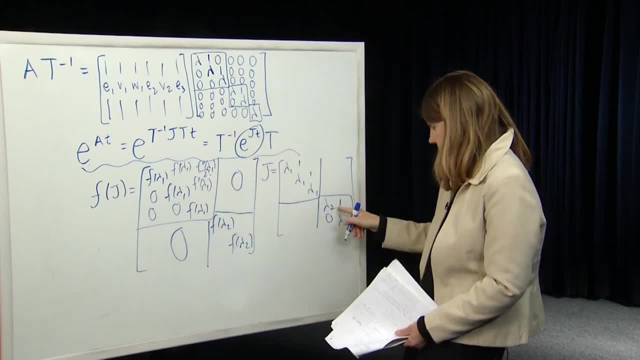 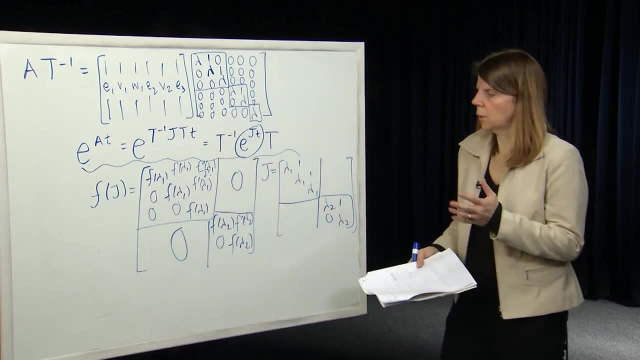 and then the only other non-zero elements are the Jordan block down here, and this is just gonna be f prime at lambda two And a zero. So this always holds: If we have a Jordan form and we have some function, f that's analytic. 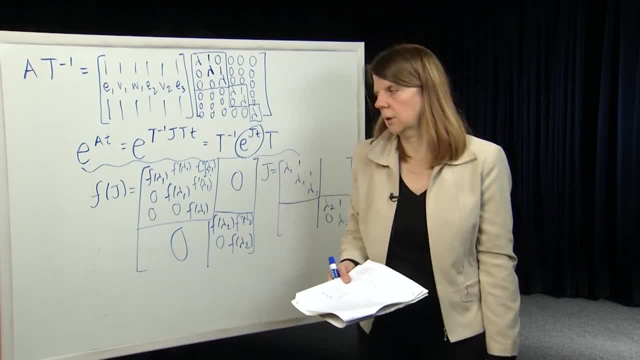 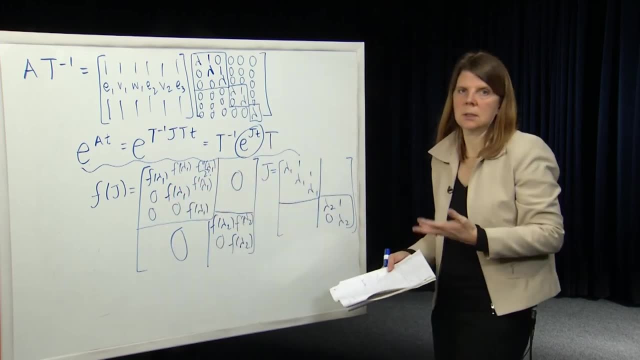 basically that means that it can be expressed locally as a polynomial around the eigenvalues of the matrix J. then we can construct given J, we can construct by inspection a function of that matrix J. So now you can take that and you can extrapolate. 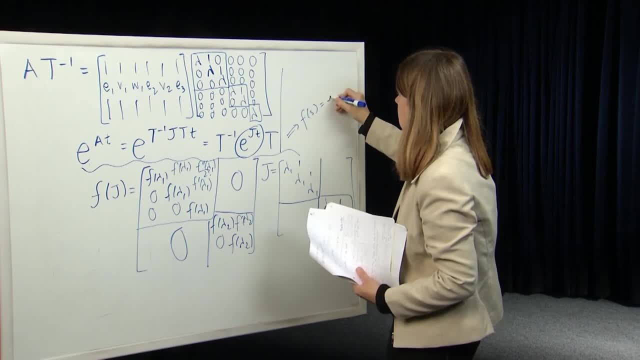 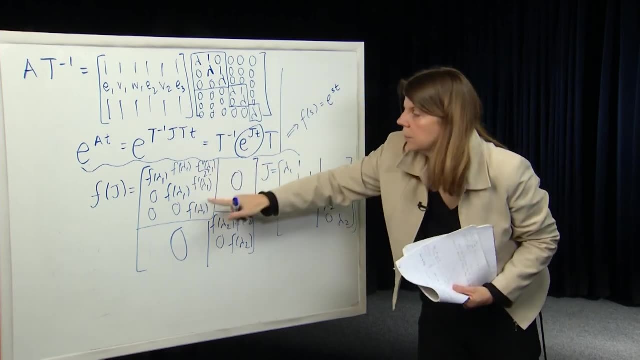 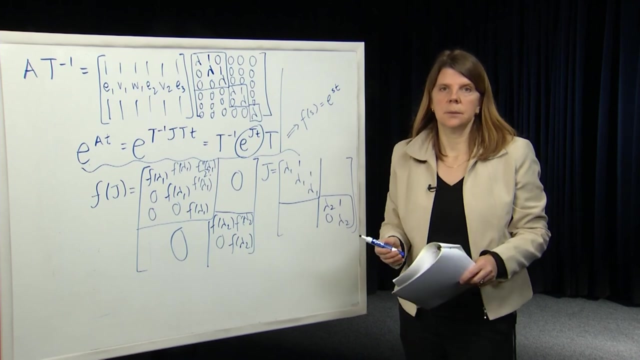 to suppose f of s is equal to e to the st, And so we take the derivative with respect to s of e to the st and we can compute this matrix e to the jt, which is what's needed eventually to compute e to the at. 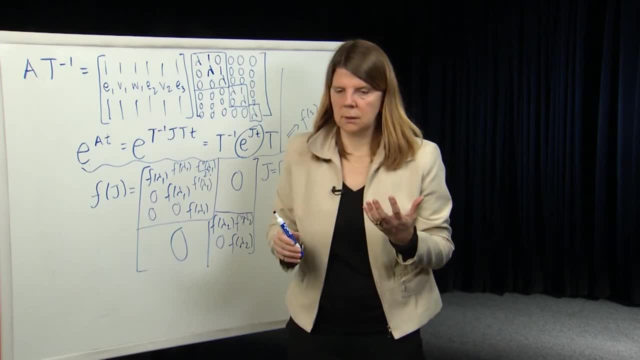 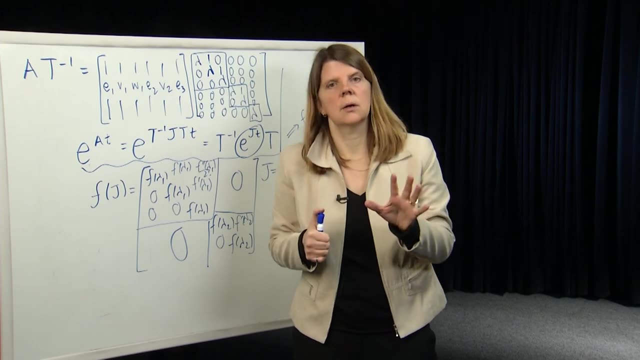 Okay, so we've now. we've talked about really two things in simplifying this computation of e to the at. We've talked about a diagonalization, which is a similarity transform in the case where we have n linearly independent eigenvectors. 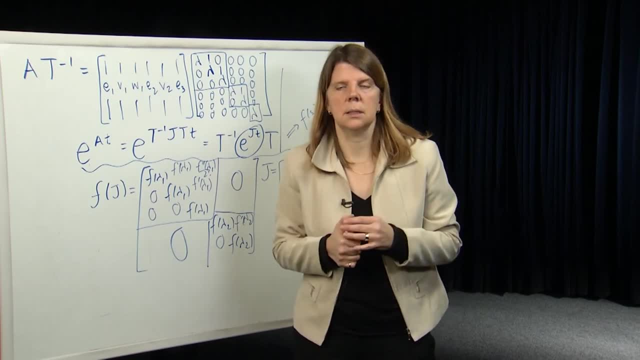 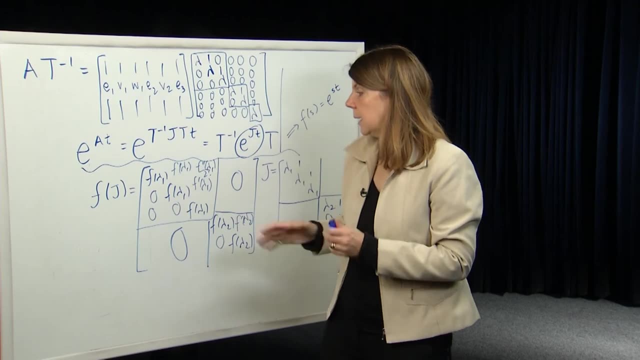 that allows us a very simple form of e to the, e to the st, And then similarly, in general, we've shown that the generalization of the diagonal form is the Jordan form and in that case also we can write down e to the at by inspection. 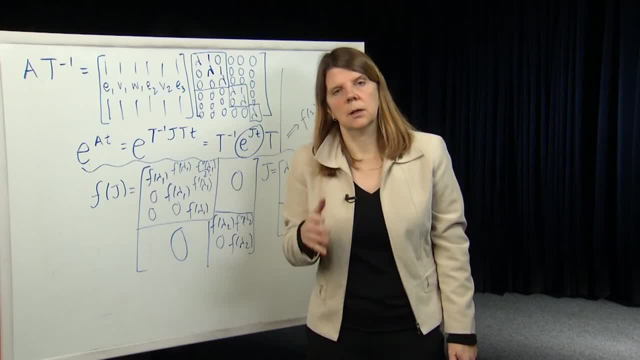 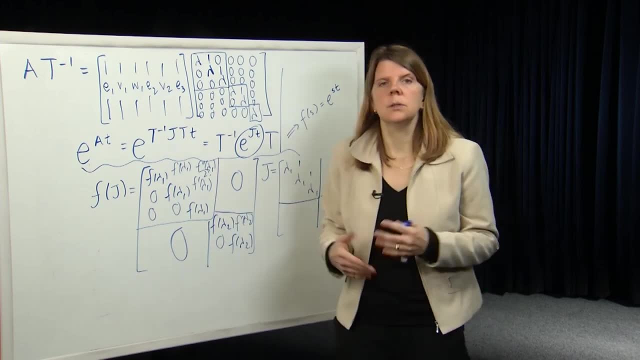 just by knowing the Jordan form, And we know how to compute the similarity transform. that takes us to the Jordan form. All right, so now we'd like to move forward and think about how we're going to use this in systems analysis, and that's the topic. of the next several modules. Thanks very much.